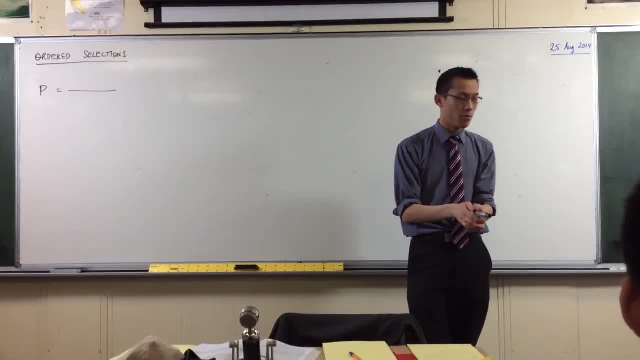 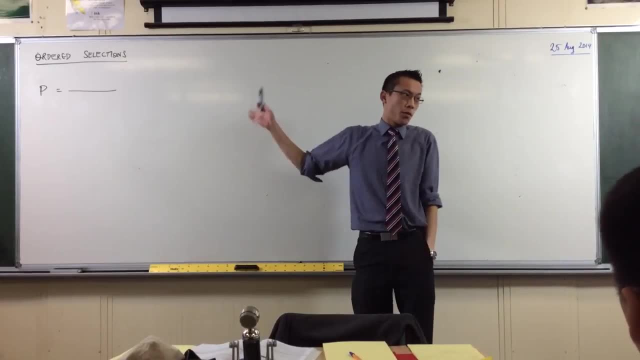 We're in the overarching topic of probability, of how likely is something to happen over another thing. what's the chance? okay, Now, we've looked at this before and we keep coming back to this fundamental idea because, simple as it is, it's full of very deep insights, right? 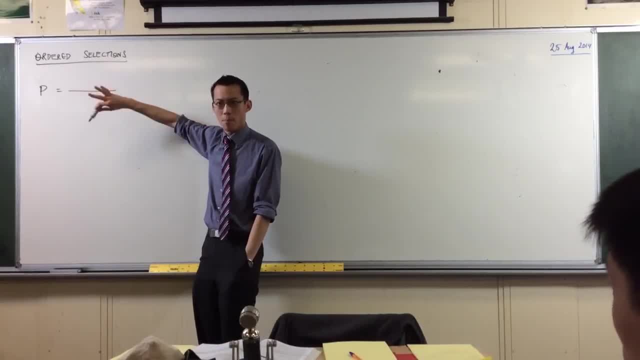 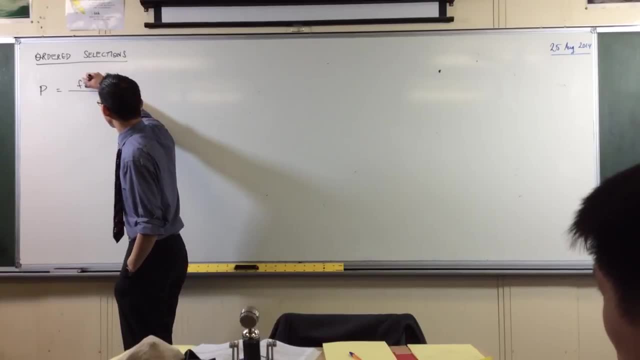 When we say probability, we mean it's a fraction, it's a comparison between two quantities, something over something. The things are on the numerator: favorable outcomes, you know, the ones that you're interested in, the ones that you want. 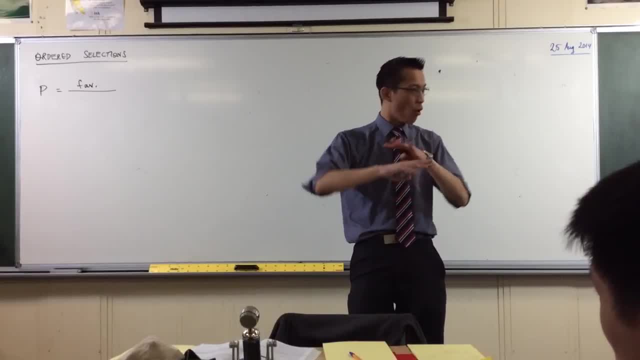 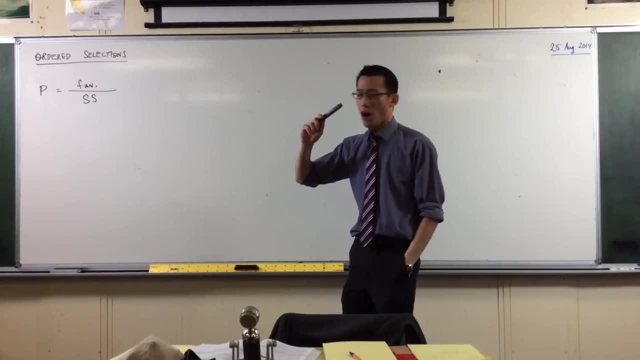 divided by the sample space, or all the total things that can happen. sample space: okay. Now one of the things that we have discovered is that often part of the trick of the question is just being able to work out what these are, but they're complicated. 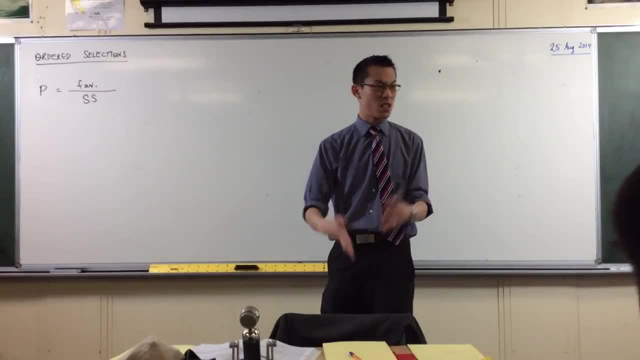 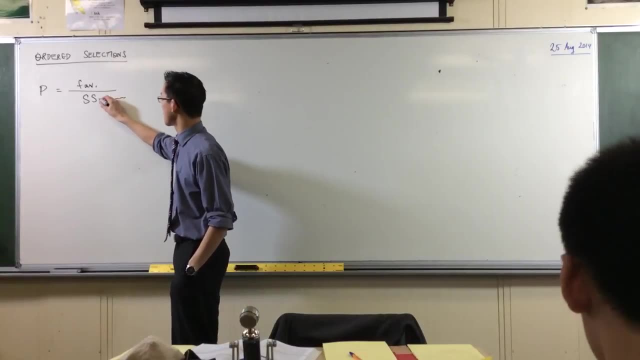 But once you get that, like all you have to do is you know, multiply the right things or simplify. Simplify easy enough, okay. So one of the most common things that we get is that you know, for example, your sample space is: I select 10 socks in a row. 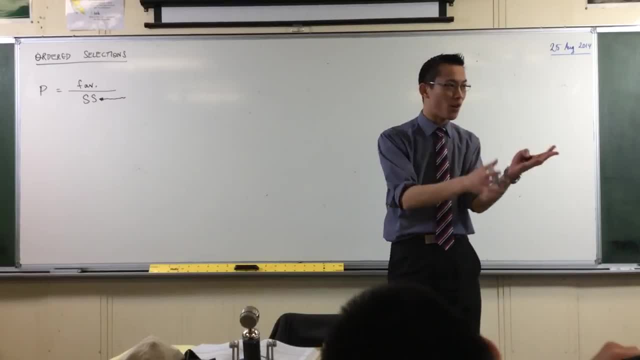 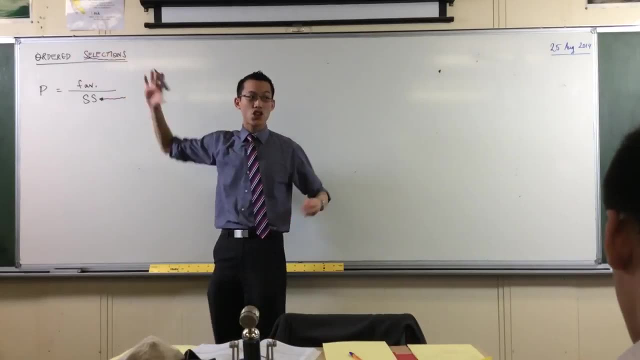 That's a sample space, right, And the order of those socks it matters because I want there to be pairs in there, right? So selecting things in a certain order is kind of half the problem of working out probabilities of different things okay. 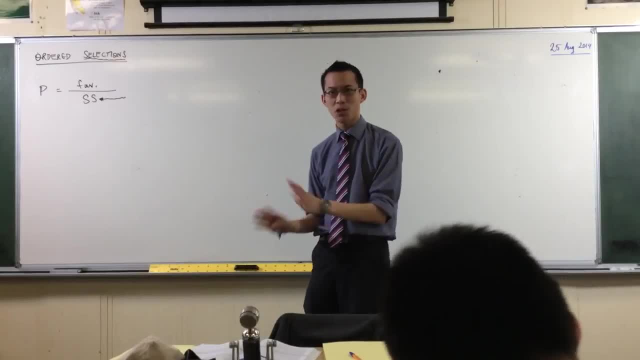 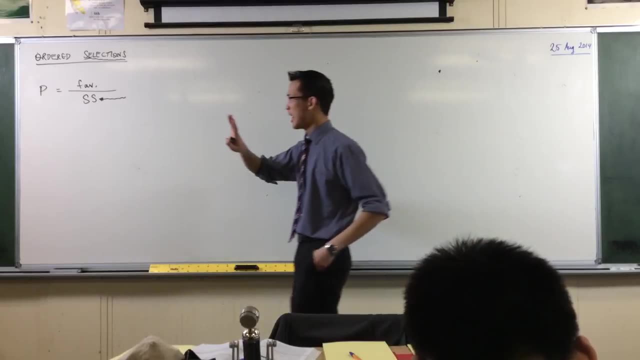 And there's a whole bunch of important things just about. So what you'll find is, as we look at it over the next couple of exercises, right, That the language of what is the chance, what is the probability, will sort of recede into the background for a little while. 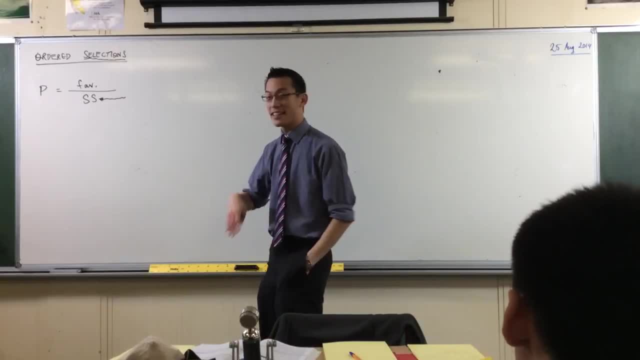 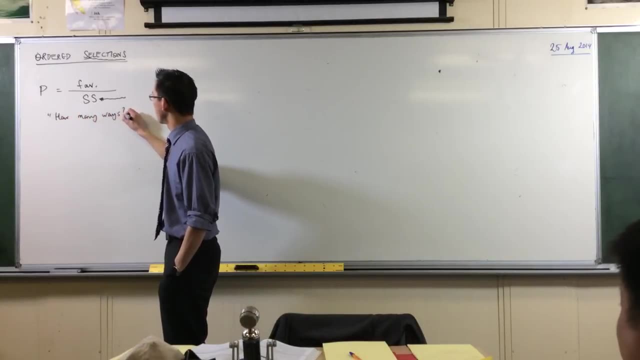 It'll go sort of on the back burner And instead you'll hear you know the phraseology of how many ways, right? So we're not working out fractions anymore, We're going to be working out numbers, Big numbers, right? 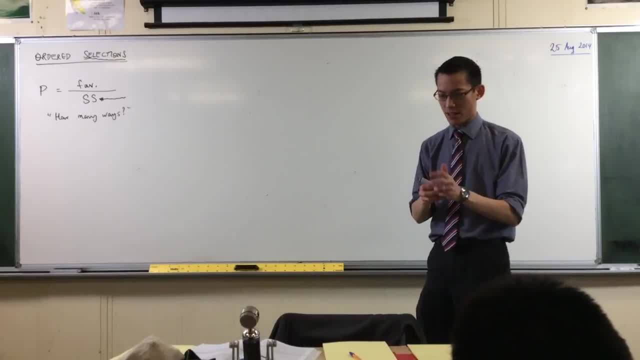 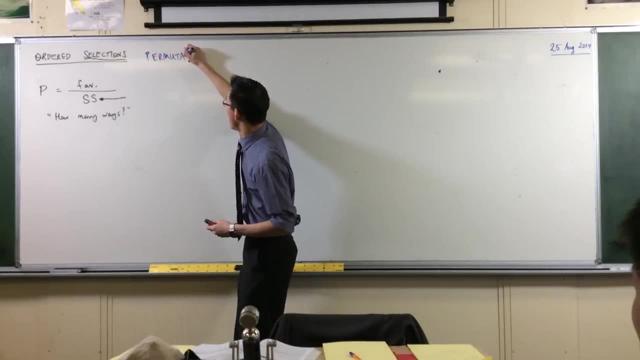 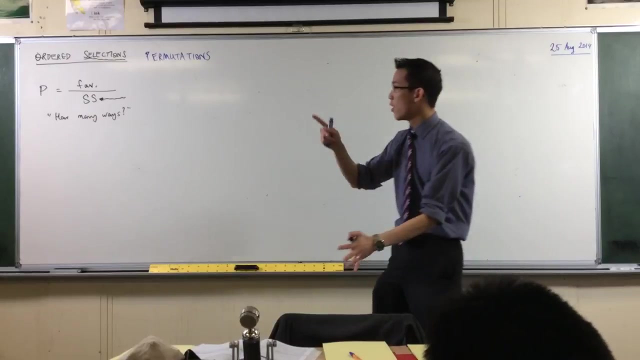 Like infinity. By the way, ordered selections- that's a bit of a mouthful. Mathematicians tried to make it a little better, but they didn't succeed very well. The other fancy name for this is permutations. okay, How many ways are there to select from a bunch of different things when you're interested in the order? 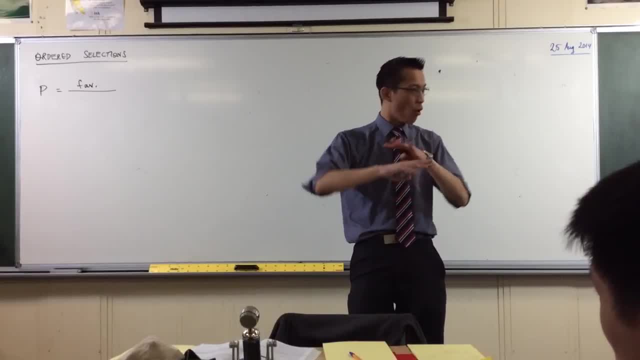 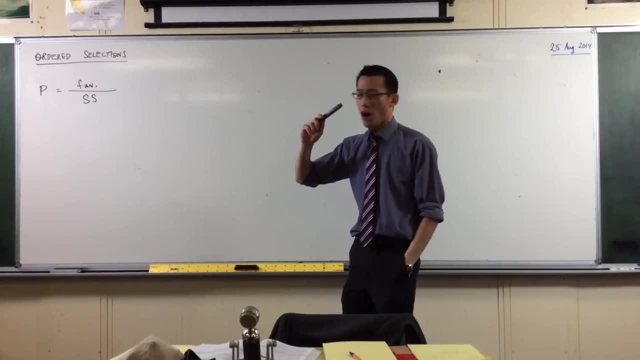 divided by the sample space, or all the total things that can happen. sample space: okay. Now one of the things that we have discovered is that often part of the trick of the question is just being able to work out what these are, but they're complicated. 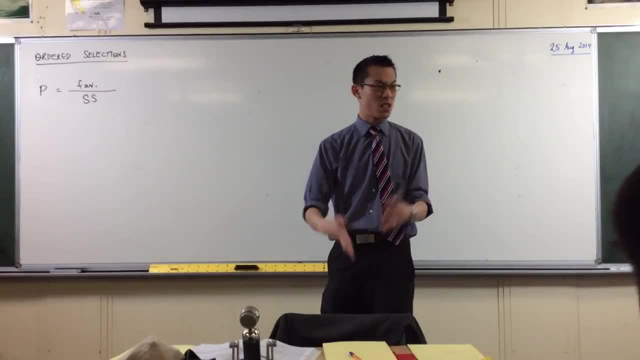 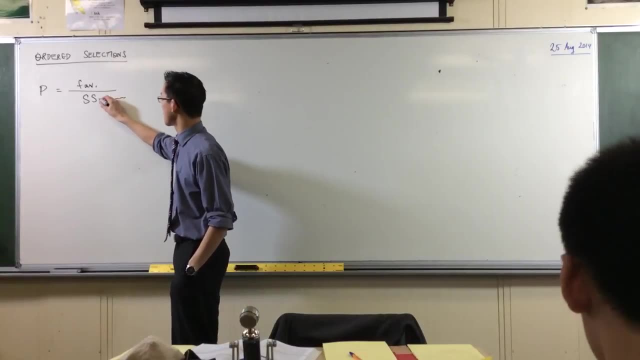 But once you get that, like all you have to do is you know, multiply the right things or simplify. Simplify easy enough, okay. So one of the most common things that we get is that you know, for example, your sample space is: I select 10 socks in a row. 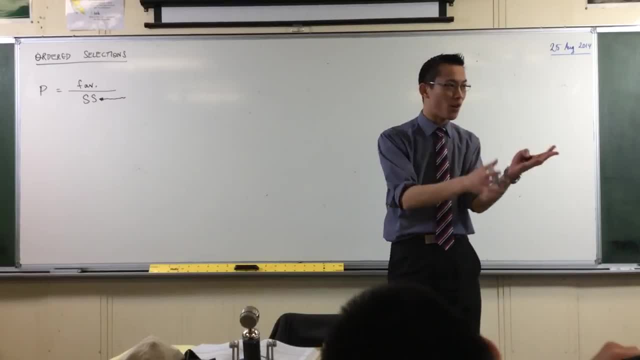 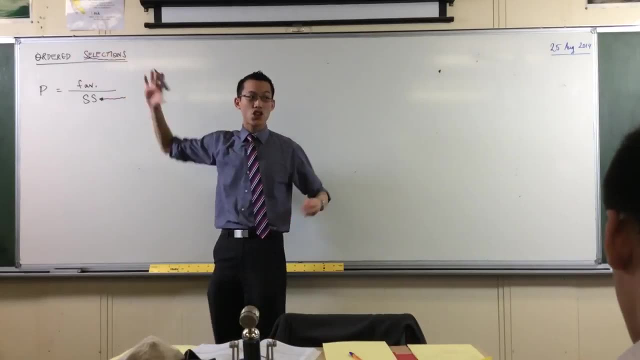 That's a sample space, right, And the order of those socks it matters because I want there to be pairs in there, right? So selecting things in a certain order is kind of half the problem of working out probabilities of different things okay. 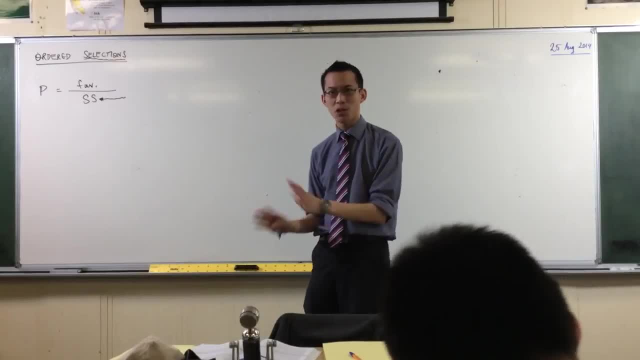 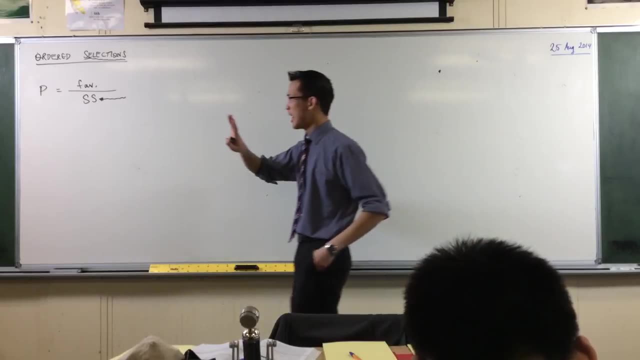 And there's a whole bunch of important things just about. So what you'll find is, as we look at it over the next couple of exercises, right, That the language of what is the chance, what is the probability, will sort of recede into the background for a little while. 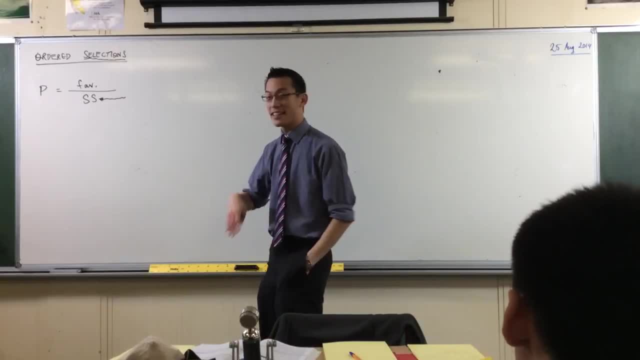 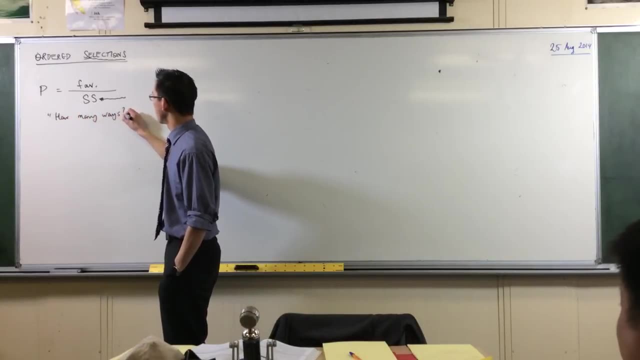 It'll go sort of on the back burner And instead you'll hear you know the phraseology of how many ways, right? So we're not working out fractions anymore, We're going to be working out numbers, Big numbers, right? 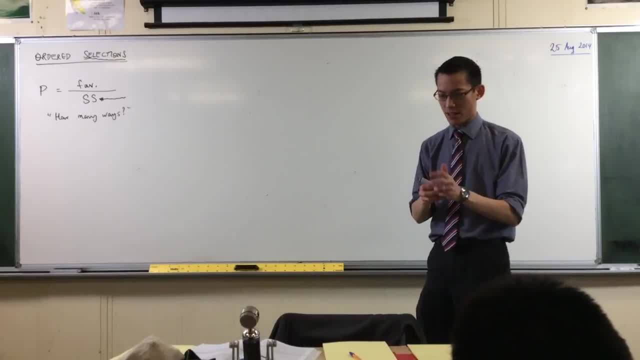 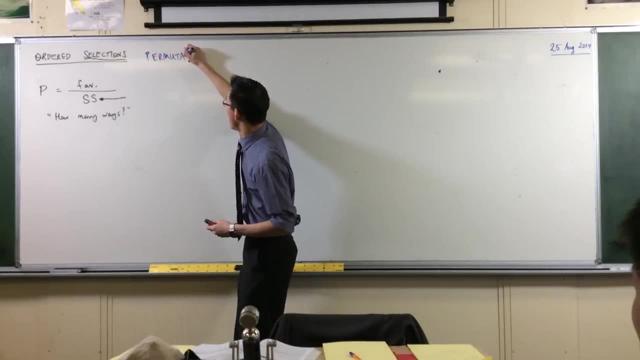 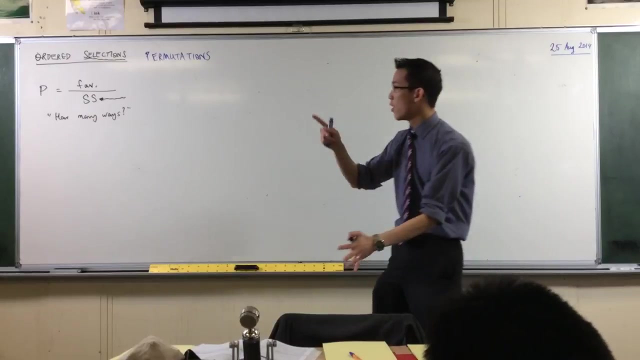 Like infinity. By the way, ordered selections- that's a bit of a mouthful. Mathematicians tried to make it a little better, but they didn't succeed very well. The other fancy name for this is permutations. okay, How many ways are there to select from a bunch of different things when you're interested in the order? 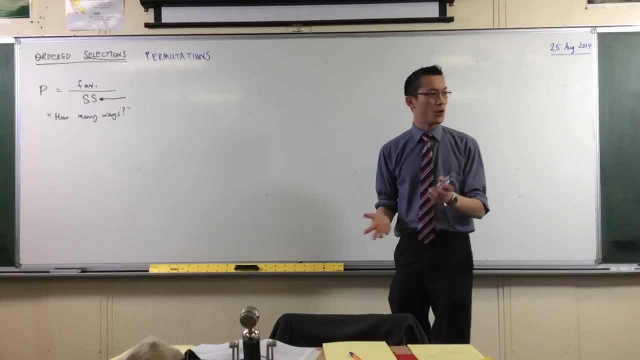 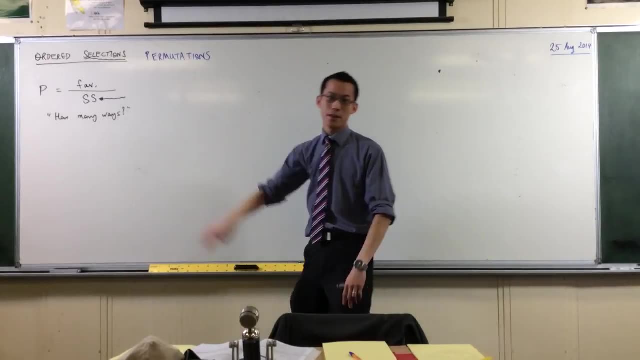 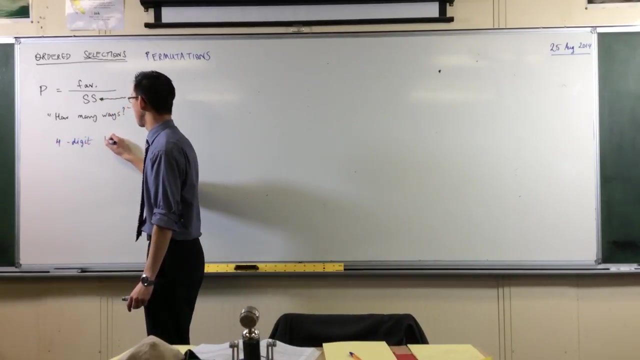 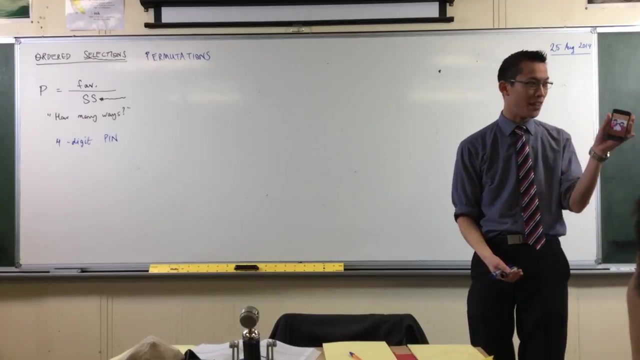 And we call those permutations okay, So you might recognize that word. Now let's look at a simple example. okay, How many permutations are there of Example, a four-digit pin? a four-digit pin, right, Because you know, if you've got a bank card or if you've got a phone that you care the security about, you're going to have a four-digit pin right. 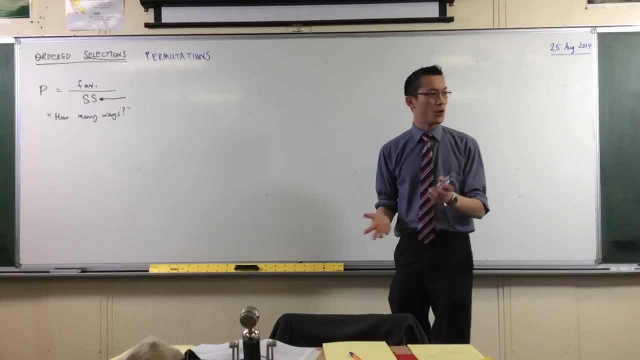 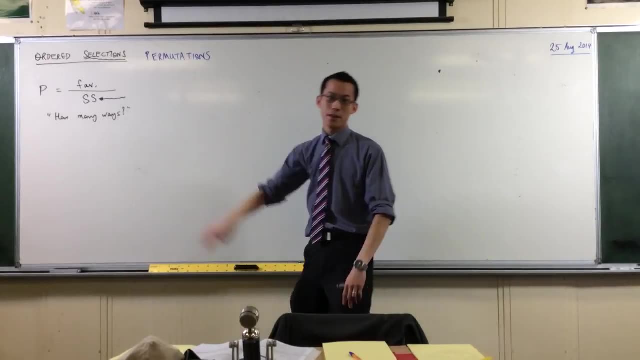 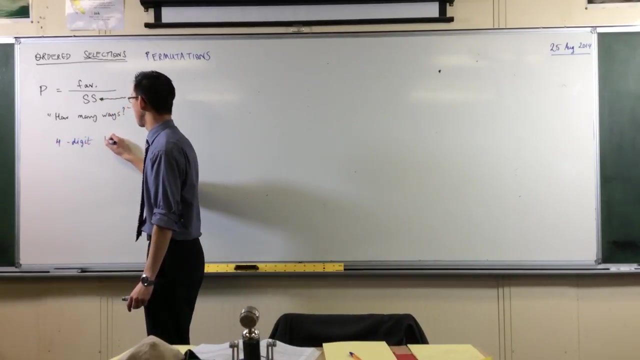 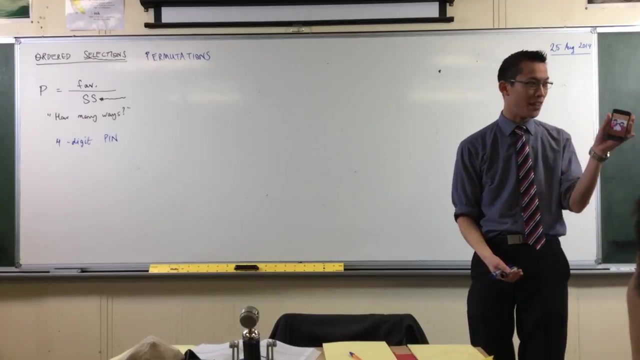 And we call those permutations okay, So you might recognize that word. Now let's look at a simple example. okay, How many permutations are there of Example, a four-digit pin? a four-digit pin, right, Because you know, if you've got a bank card or if you've got a phone that you care the security about, you're going to have a four-digit pin right. 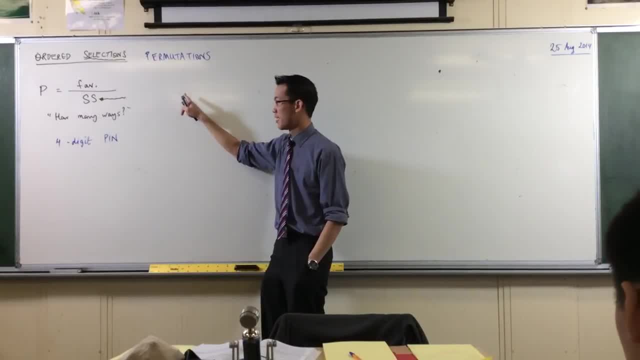 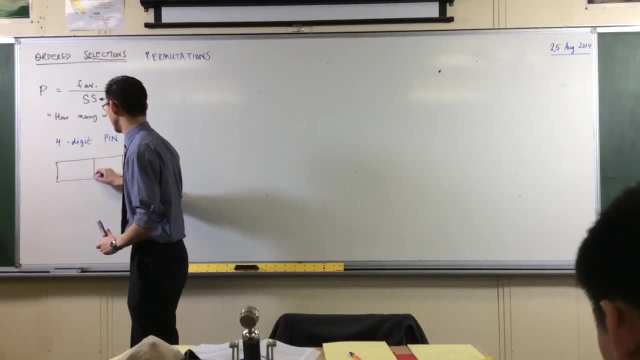 Well, how many different ways, how many permutations can you get of this thing? okay? Well, let's think about it like this: Here are some questions. Here are the slots where my four-digit pin is going to go. okay, In fact, that's what my screen even looks like. 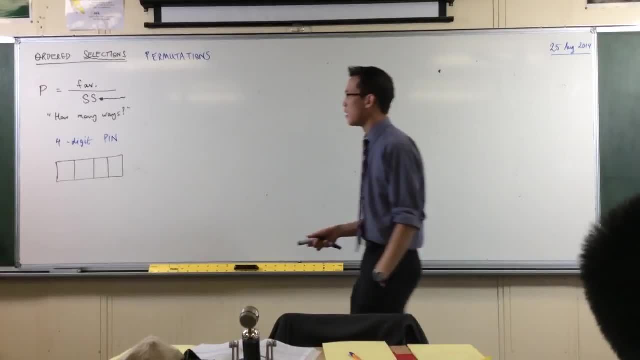 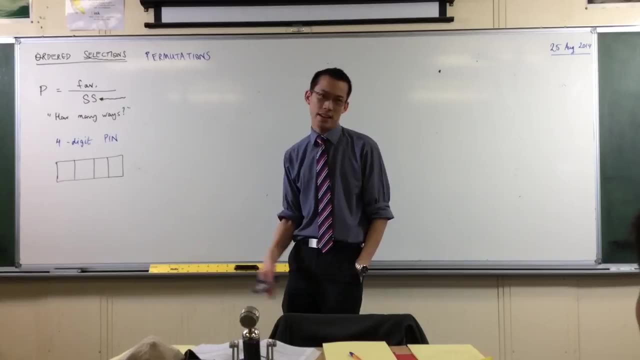 Turn it on. it's like, look, you're going to have to type in four characters. okay, Now you then think about what's going to go in each of these slots. right Now, if I say four-digit, like let's stick with numbers. 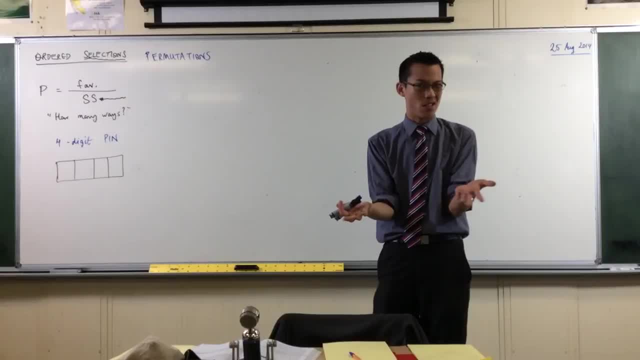 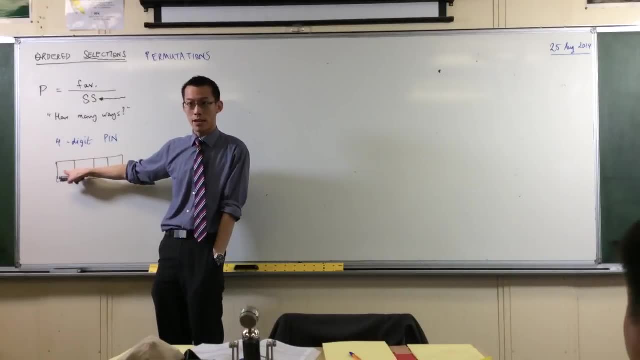 You know, if you go to the shops in the EFTPOS machine it's just got numbers on it. really, How many options have I got to put into? you know you're making a password into this first spot over here. 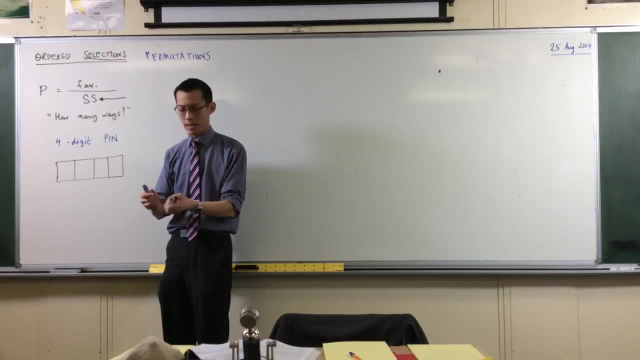 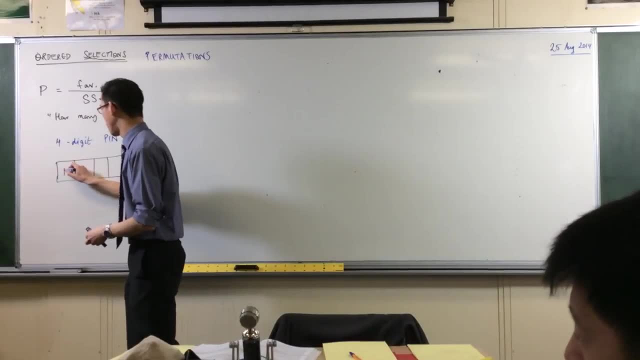 One, Two, Three, Four, Five, Six. Now I count the options as zero: one, two, three, four, five, six, seven, eight, nine. right, So I have ten options. right, So I can put ten different things in that spot. 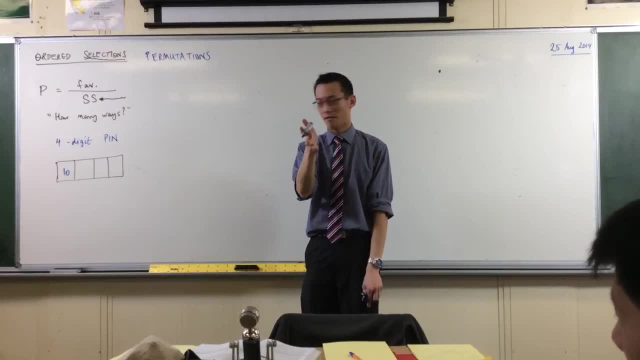 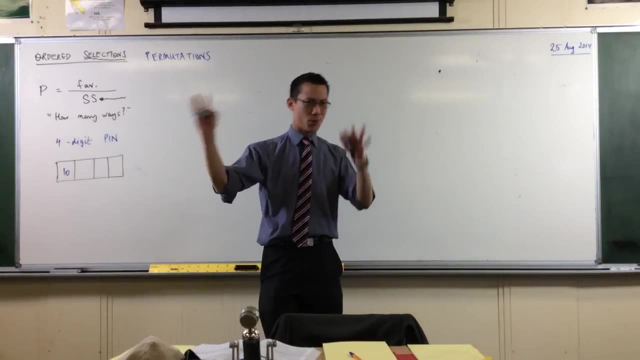 Cool Now when I move it over to the next spot, right, So this is like a multi-stage event. if you like, I've got another ten options I don't have to worry about, you know, with or without replacement or anything. 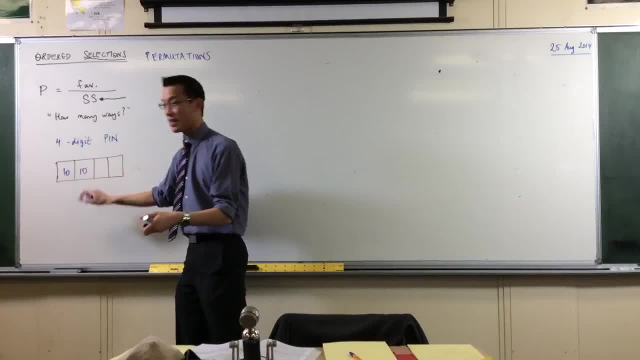 I'm just picking a number, that's all okay. So I've got another ten different options, and then another ten, and then another ten, Easy right. So, being that I have to pick all four and they all combine together, 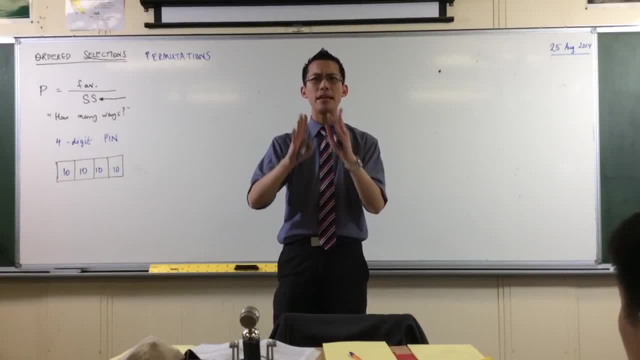 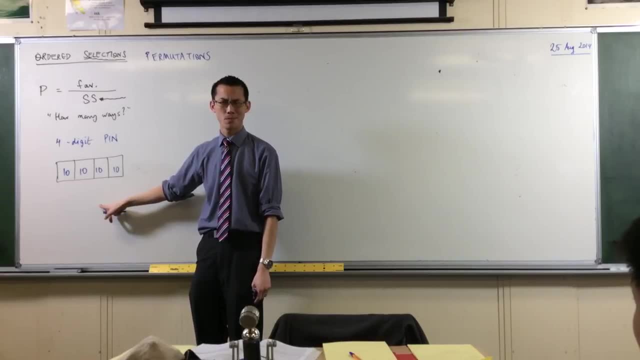 remember, it's a multi-stage event, but this is all happening simultaneously. It's one event. So what do I do with these numbers? Which rule do I use? This is the product rule, isn't it? Because all of these characters' events happen at the same time. to make my four-digit pin. 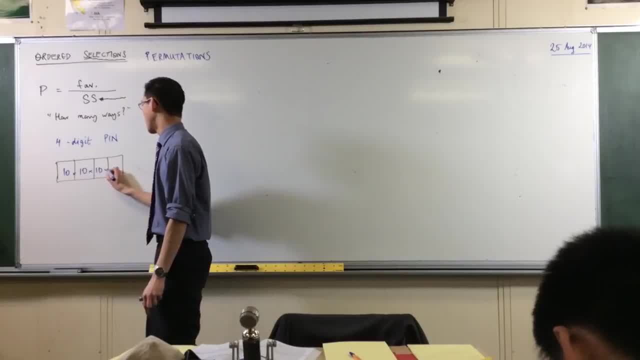 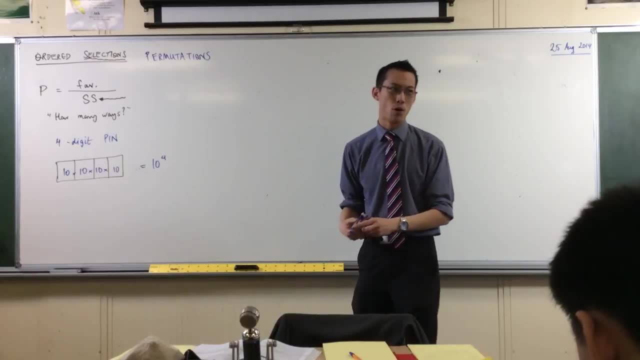 So I multiply them, I get ten times ten times ten times ten. So there are ten to the four different combinations And you can see very easily how this could turn into a probability question, right? For instance, if I randomly pick up your phone and try and guess your password. 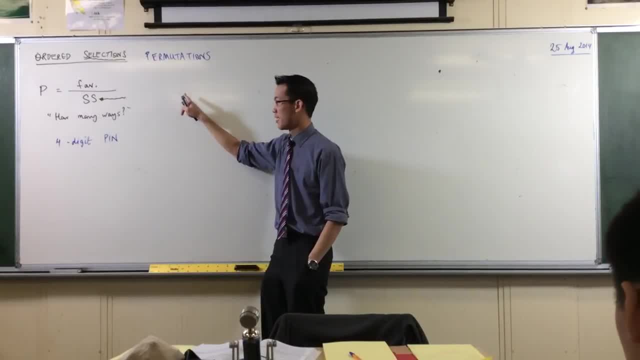 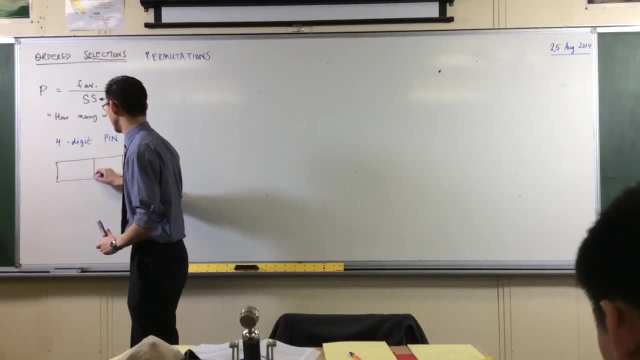 Well, how many different ways, how many permutations can you get of this thing? okay? Well, let's think about it like this: Here are some questions. Here are the slots where my four-digit pin is going to go. okay, In fact, that's what my screen even looks like. 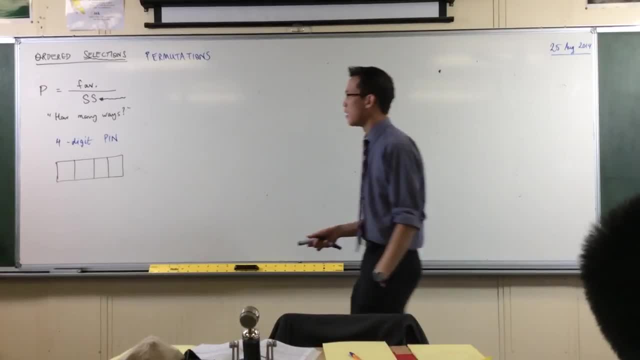 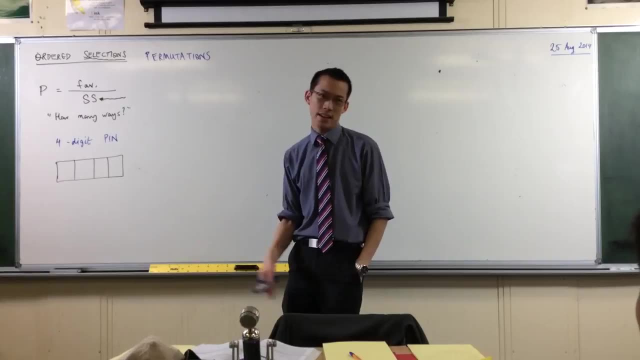 Turn it on. it's like, look, you're going to have to type in four characters. okay, Now you then think about what's going to go in each of these slots. right Now, if I say four-digit, like let's stick with numbers, you know, if you go to the shops in the EFTPOS machine it's just got numbers on it. really, 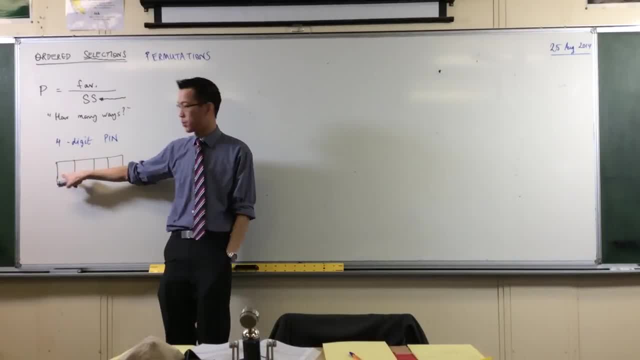 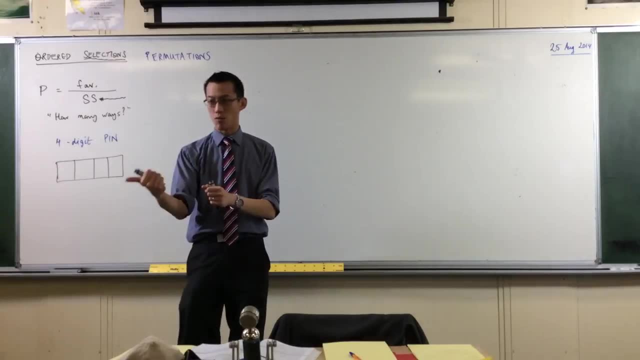 How many options have I got to put into? you know you're making a password into this first spot over here. Hmm, now I count the options as zero, one, two, three, four, five, six, seven, eight, nine, right. 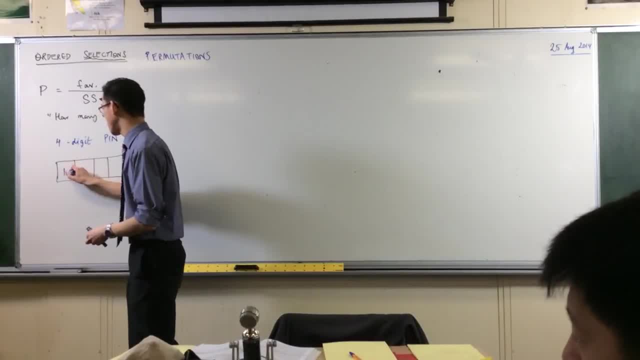 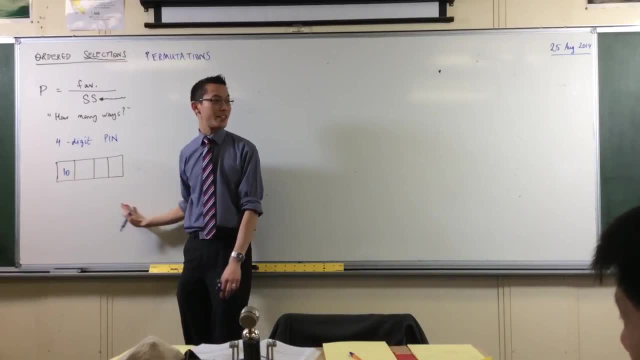 So I have ten options, right, So I can put ten different things in that spot. cool. Now when I move it over to the next spot, right? So this is like a multi-stage event, if you like. 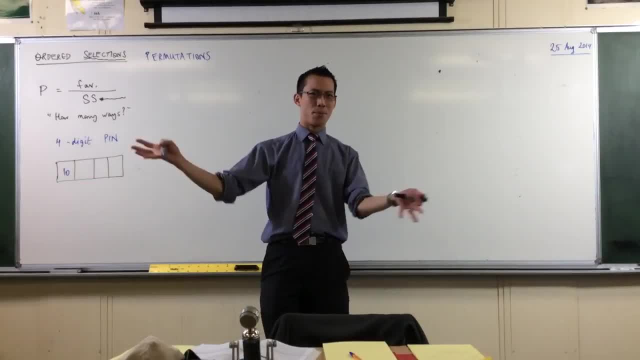 I've got another ten options. I don't have to worry about, you know, with or without replacement or anything, I'm just picking a number. that's all okay. So I've got another ten different options and then another ten. 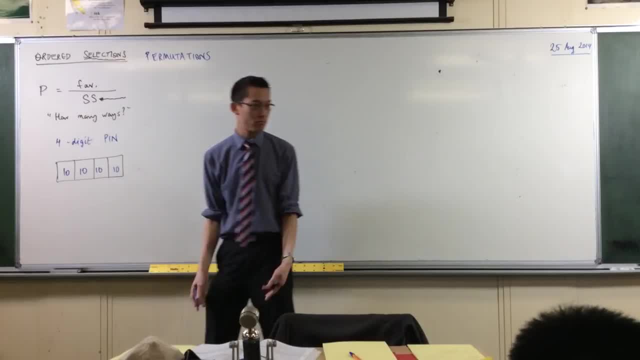 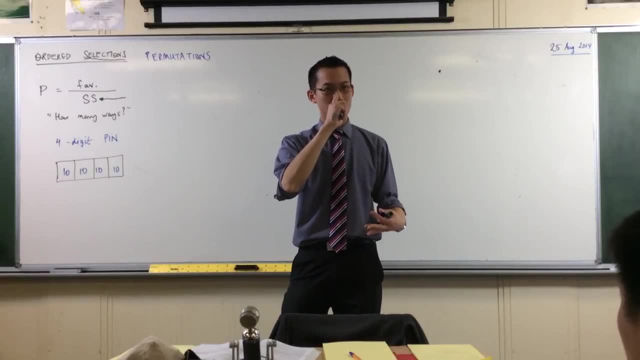 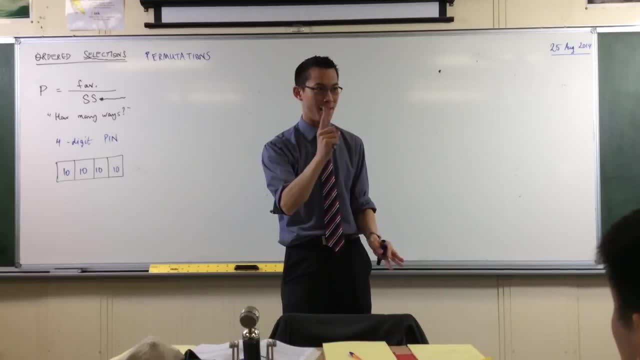 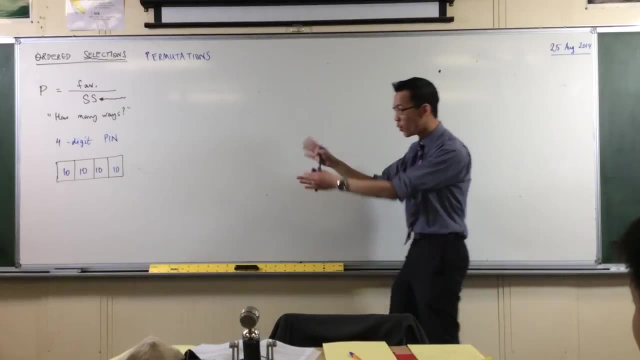 but this is all happening simultaneously. It's one event. So what do I do with these numbers? Which rule do I use? This is the product rule, isn't it? Because all of these characters' events happen at the same time to make my four-digit pin? 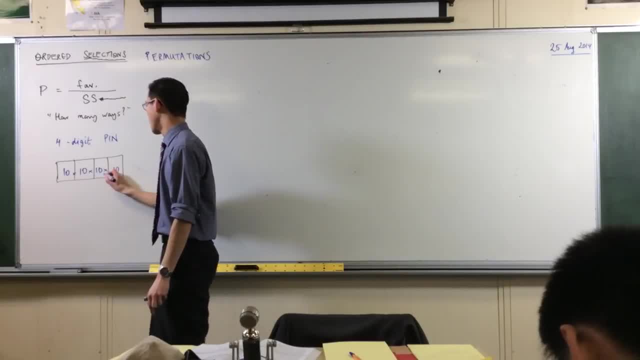 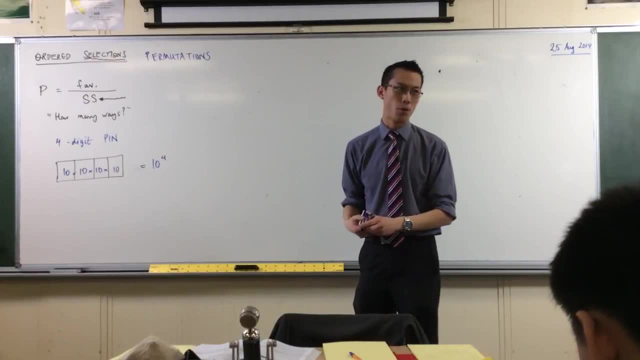 So I multiply them, I get ten times ten times ten times ten. So there are ten to the four Different combinations And you can see very easily how this could turn into a probability question, right? For instance, if I randomly pick up your phone and try and guess your password. 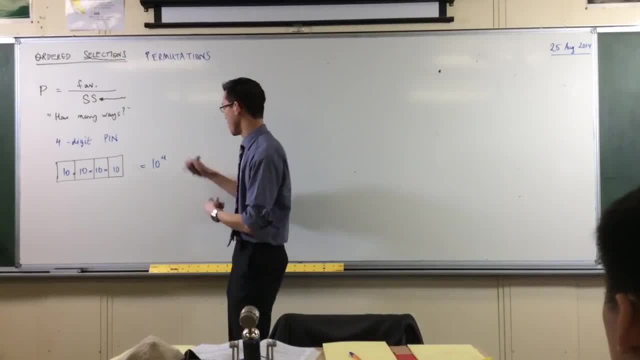 what is the probability that I guess the right password? And the answer is, you know, one in ten thousand. Not very good chances, right, But there you go. You can see how this question feeds into this question. Make sense, Okay? 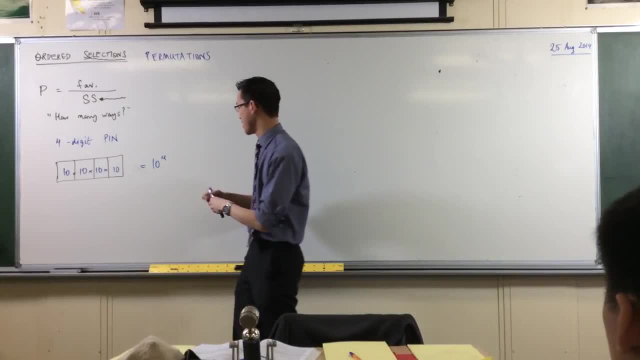 what is the probability that I guess the right password? And the answer is, you know, one in ten thousand. Not very good chances, right, But there you go. You can see how this question feeds into this question. Make sense, Okay? 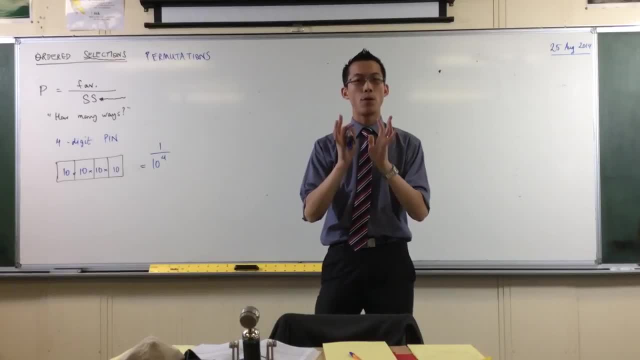 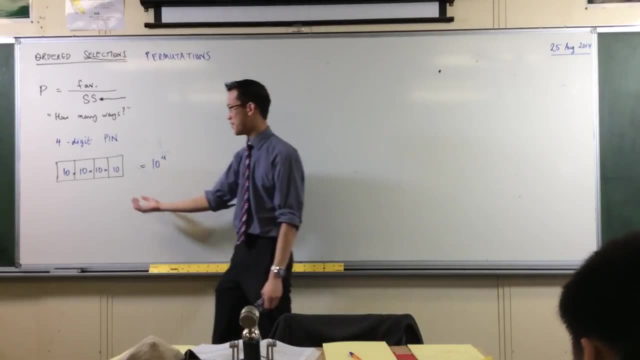 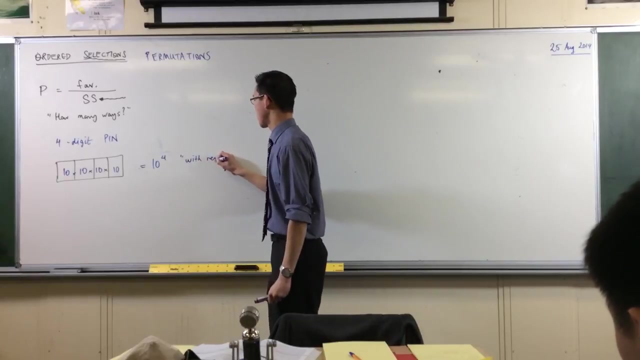 So, if you want to catch it in the language that we've already been using, okay, this thing here is with replacement. With replacement because I have the same bunch of numbers and I keep on putting it back. Okay, So this is with replacement. 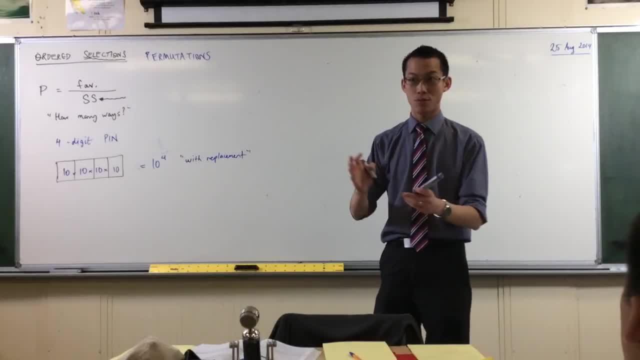 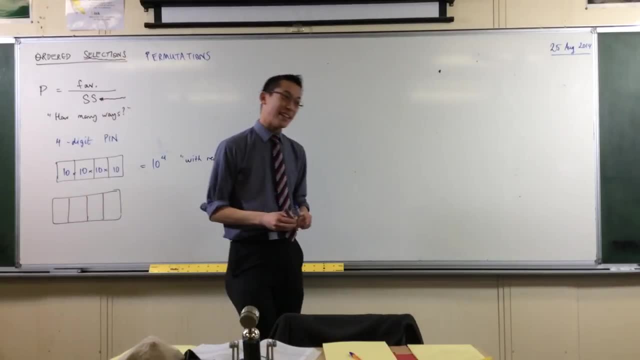 Okay Now, I know it's a little bit contrived, but let's replay the scenario. I still want a four-digit pin. Okay, But let's suppose you know I'm a bit of a. I know that repeated digits are actually a bad idea in a password. 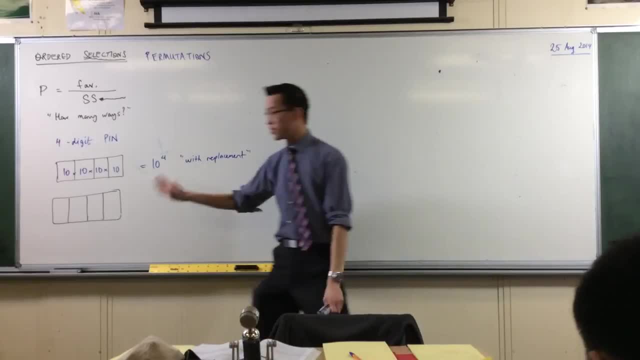 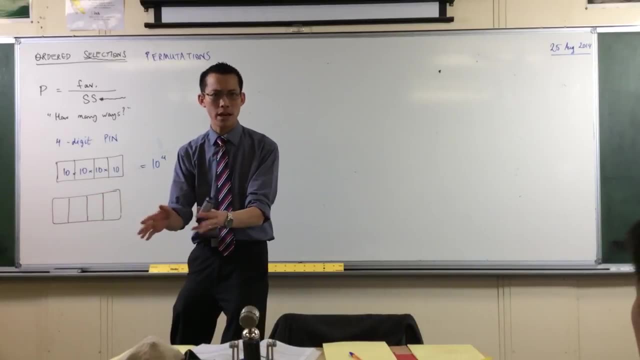 They are. So I say, look, I want to not have any repeated digits as I go through. Okay, So when I have a look at this first one, I've got all ten to pick from. Yeah, I can still pick any of zero, one, two, three, four, five, six, seven, eight, nine. 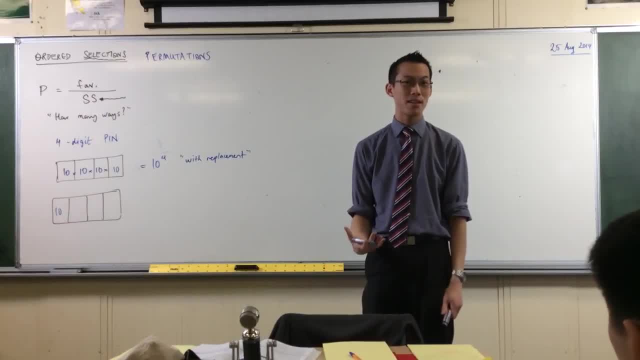 So far, so good, But then when I pick the next one, I don't want to pick from the same number. So, if you like, this is without replacement, Right. So how many options do I have left for the next number? 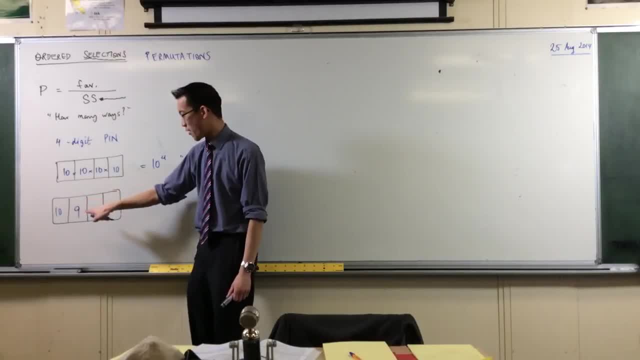 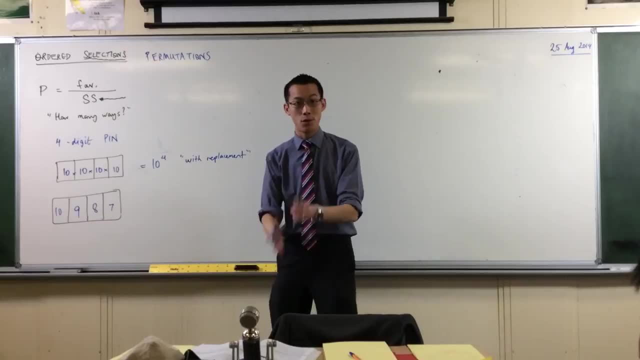 It's a nine, And then once I pick two, well, there are eight left, And then for the last one, there will be seven left. Yes, Just like before, all of these things are happening simultaneously. So again, I use the product rule. 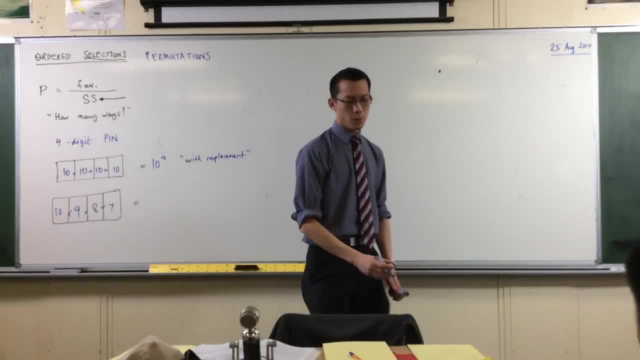 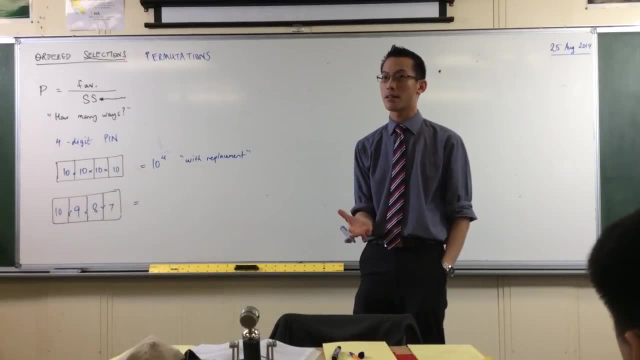 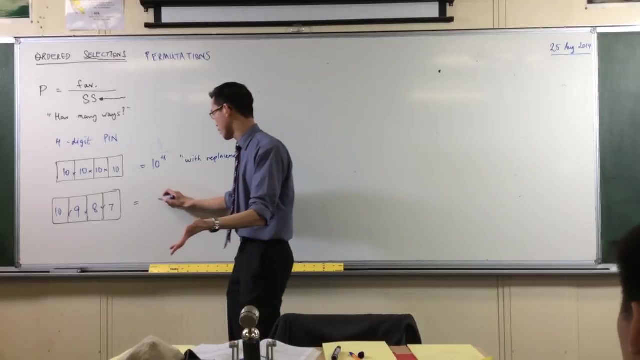 I multiply Right Now. how can we write this? How can we write this? Obviously, I can write it as just ten times nine times eight times seven, But we have language that would make this a little more concise. Right, When you're multiplying and you're decreasing by one, the language that we use is factorial notation. 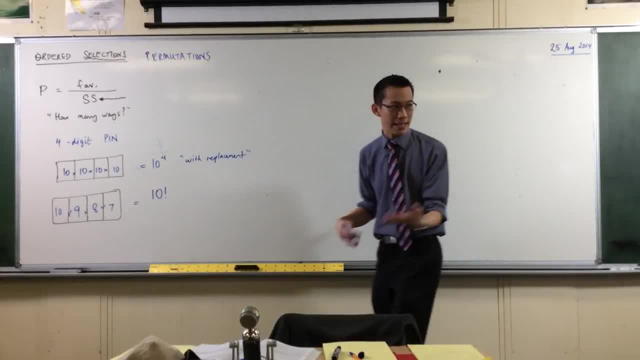 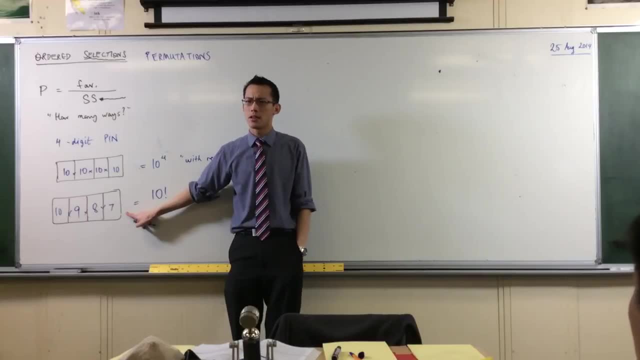 Right. So this clearly looks like ten factorial. At least it starts that way, But it doesn't end that way, It doesn't? And we looked at this under binomial Right. I'm missing. What am I missing off the end? 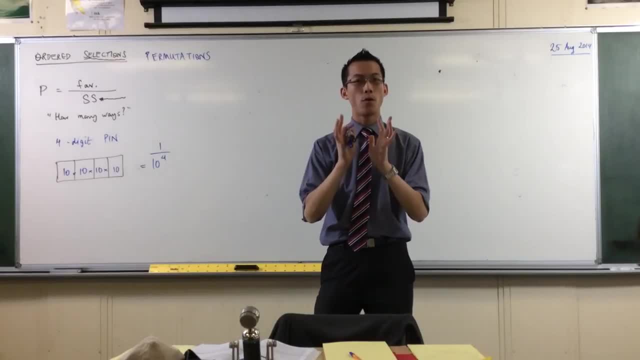 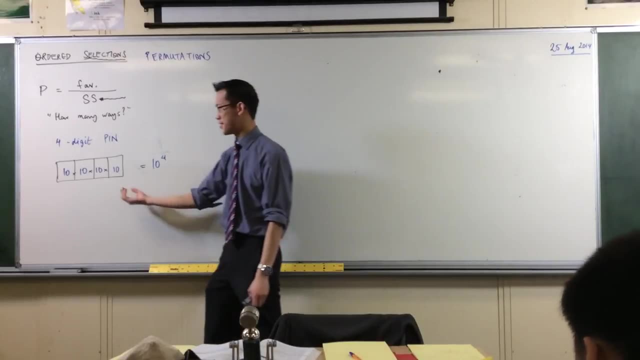 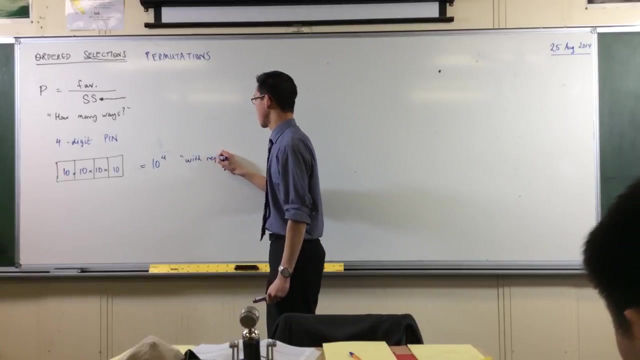 So, if you want to catch it in the language that we've already been using, okay, this thing here is with replacement. With replacement because I have the same bunch of numbers and I keep on putting it back. okay, So this is with replacement. okay, 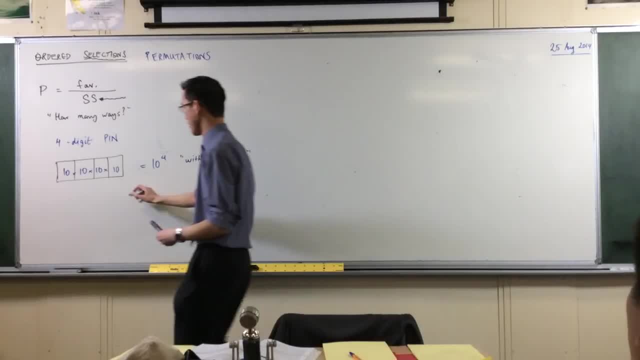 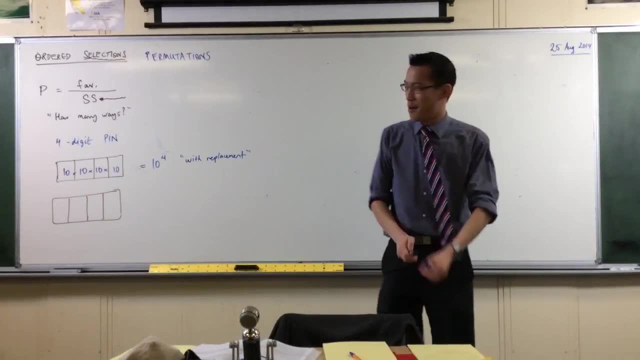 Now, I know it's a little bit contrived, but let's replay the scenario. I still want a four-digit pin. okay, But let's suppose you know I'm a bit of a. I know that repeated digits are actually a bad idea in a password. 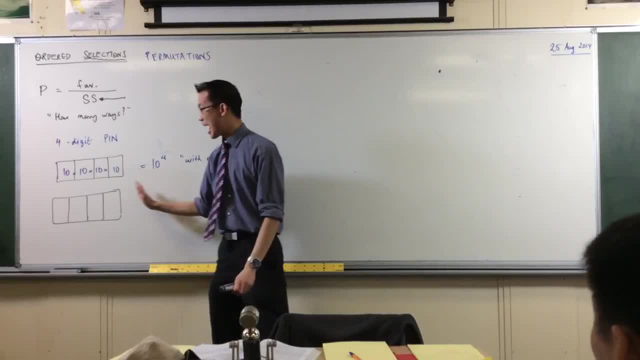 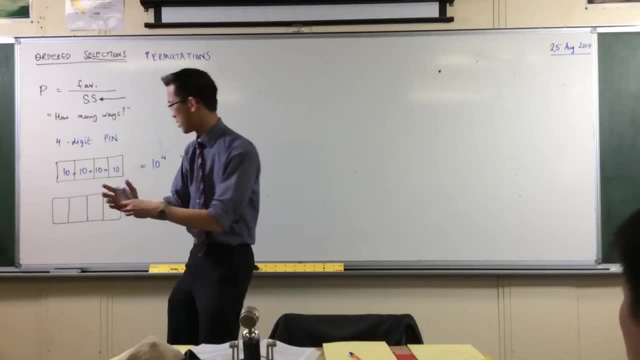 They are. So I say, look, I want to not have any repeated digits as I go through. okay, So when I have a look at this first one, I've got all ten to pick from. yeah, I can still pick any of zero, one, two, three, four, five, six, seven, eight. 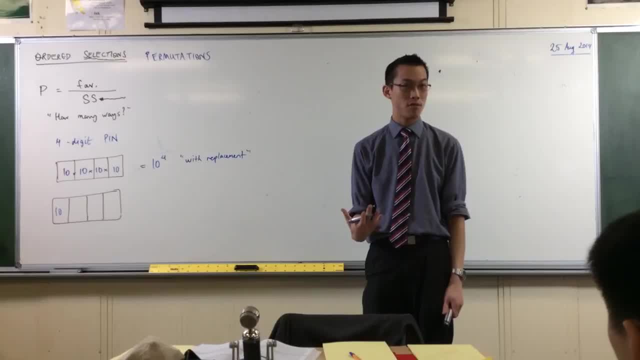 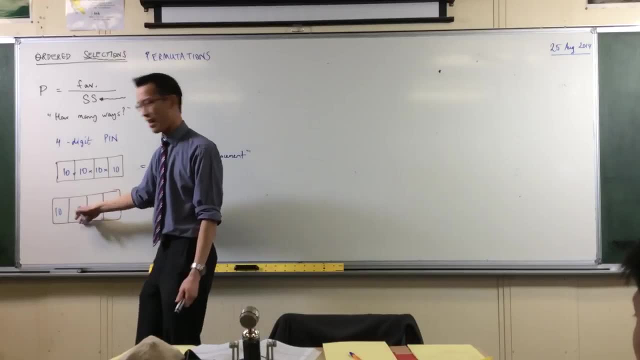 So far, so good, But then when I pick the next one, I don't want to pick from the same number. So, if you like, this is without replacement right. So how many options do I have left for the next number? 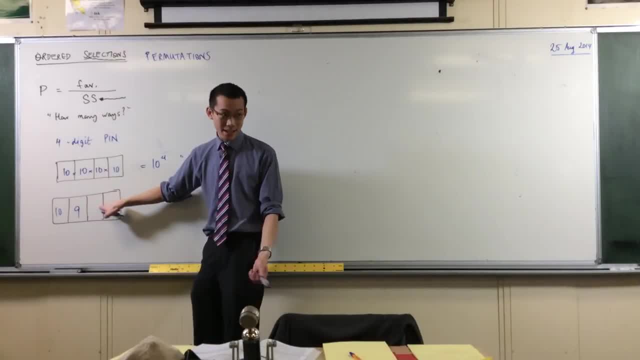 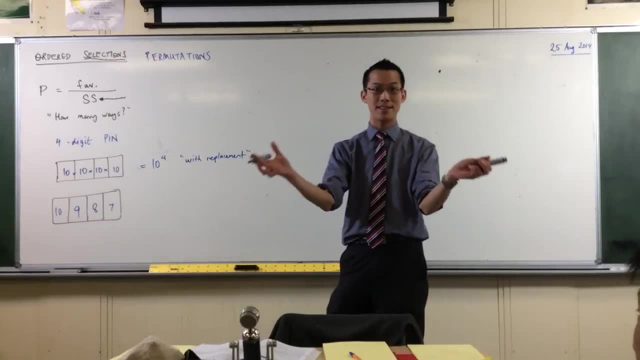 It's a nine, And then, once I pick two, well, there are eight left, And then for the last one, there will be seven. There will be seven left. yes, Just like before, all of these things are happening simultaneously. 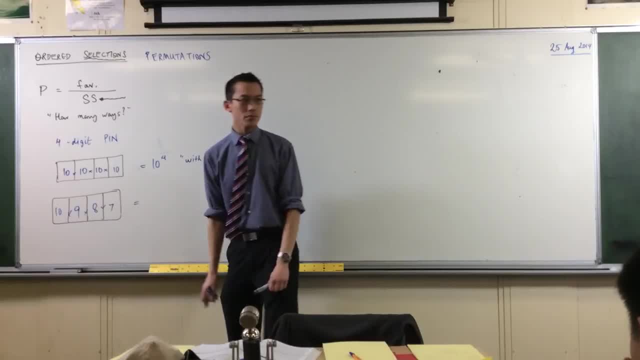 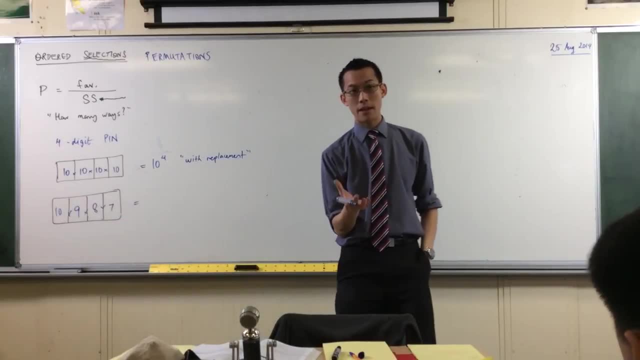 So again, I use the product rule. I multiply right Now. how can we write this? How can we write this? Obviously, I can write it as just ten times nine times eight times seven, But we have language that would make this a little more concise, right. 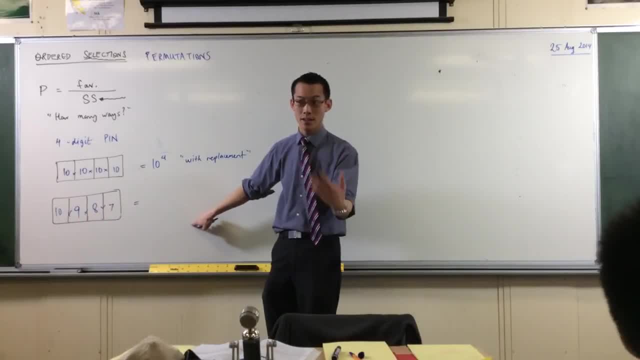 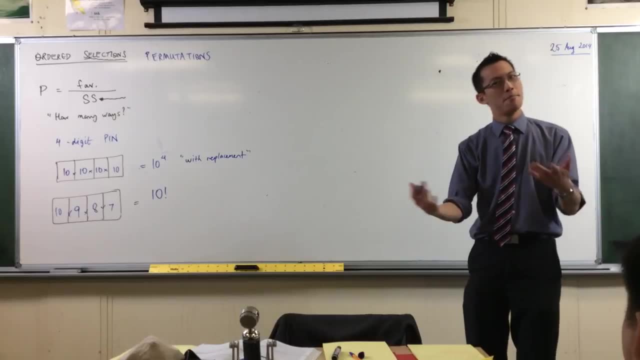 When you're multiplying and you're decreasing by one. the language that we use is Factorial notation, right? So this clearly looks like ten factorial, At least it starts that way, But it doesn't end that way, does it? 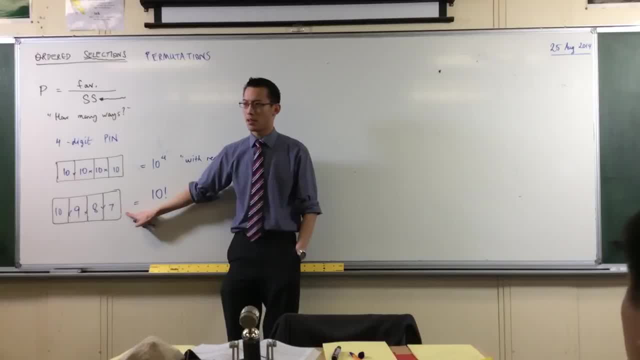 And we looked at this under binomial right. I'm missing. what am I missing off the end? I'm missing six factorial right. So you don't subtract it, though You're dividing by six factorial okay. Now I want to push on this a little further. 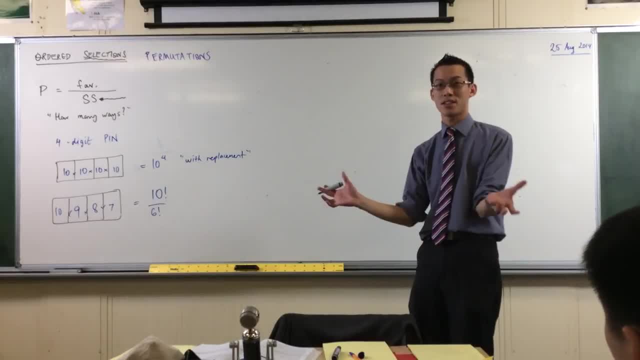 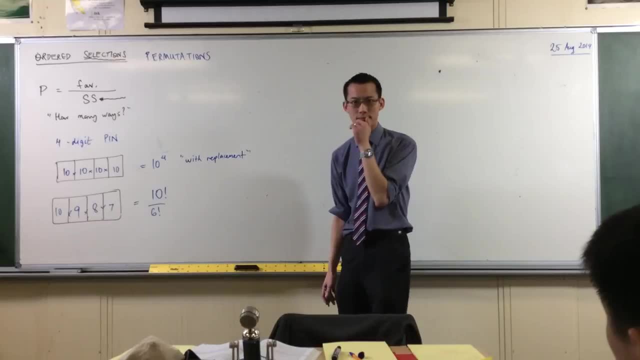 Clearly that six factorial is not just some random. I just pick out six, right? Why is it six and not seven or three? Where does that six come from? It comes from the fact that I've used four of the options, right. 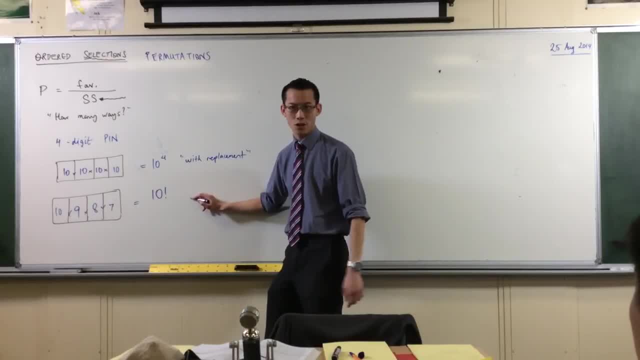 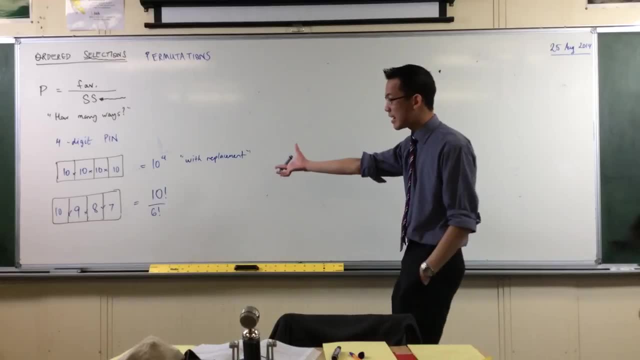 I'm missing six factorial Right, So you don't subtract it, though You're dividing by six factorial. Okay, Now I want to push on this a little further. Clearly, that six factorial is not just some random, I just pick out six. 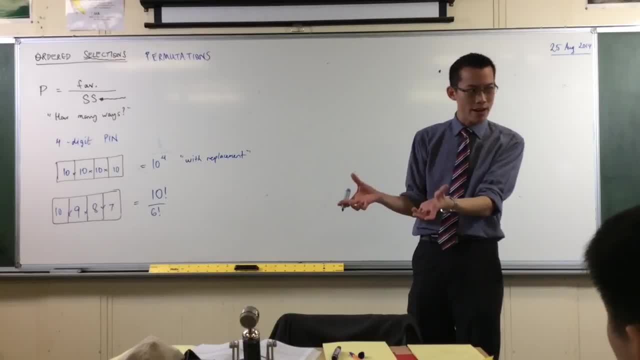 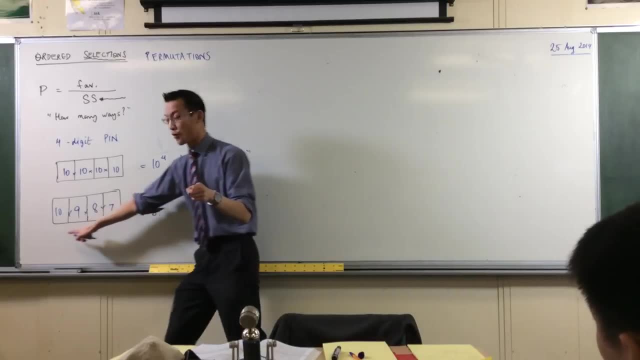 Right. Why is it six and not seven or three? Where does that six come from? It comes from the fact that I've used four of the options Right, So that's why there are six factorial left over here that I haven't included. 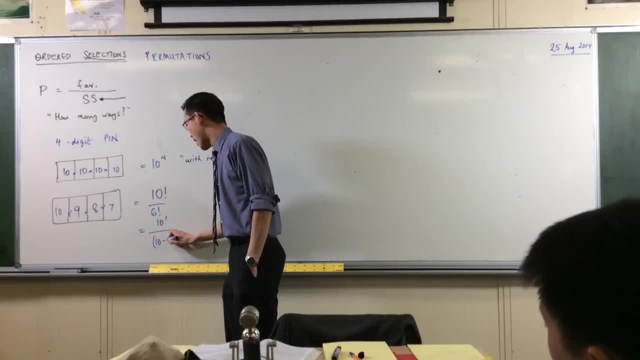 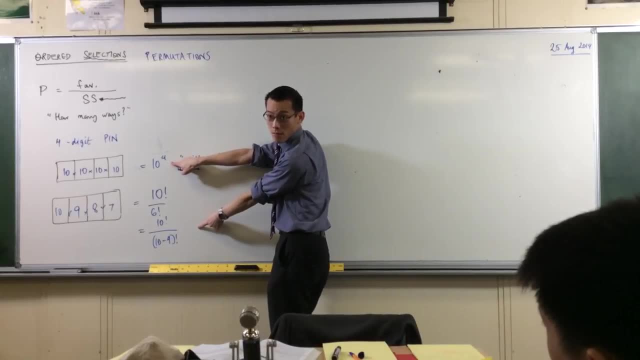 Right. So it's ten factorial on ten minus four factorial. That's really where the numbers come from And you can see it's built of the same numbers as this Right, The ten, as in how many digits there were. 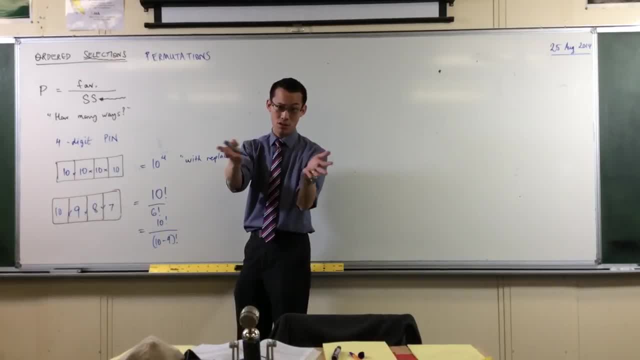 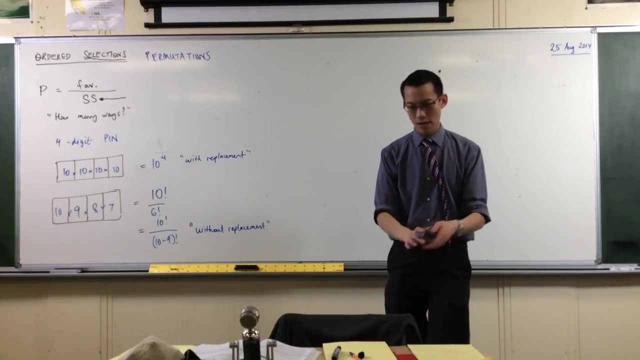 And the four, Sorry, Ten, how many different numbers you could choose from. And four, how many digits there were. That's how we built this number of permutations. Okay, So this is without replacement. Okay, So let's generalize a little bit. 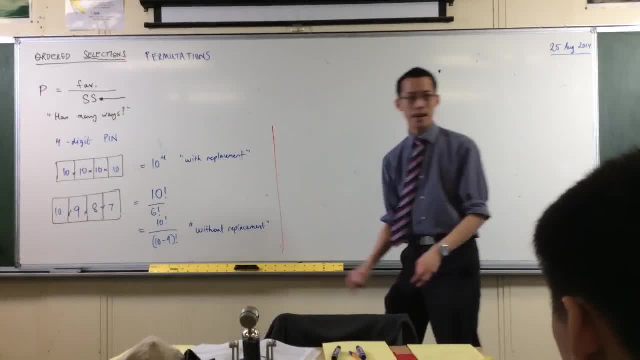 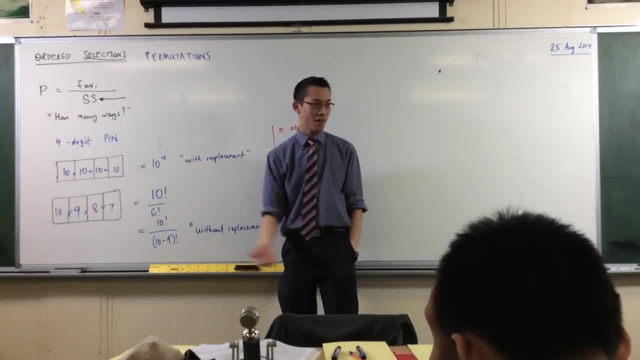 If I have, Let's put it over here, Okay- If I have n objects. N objects, For instance, if I have ten numbers Zero: one, two, three, four, five, six, seven, eight, nine. 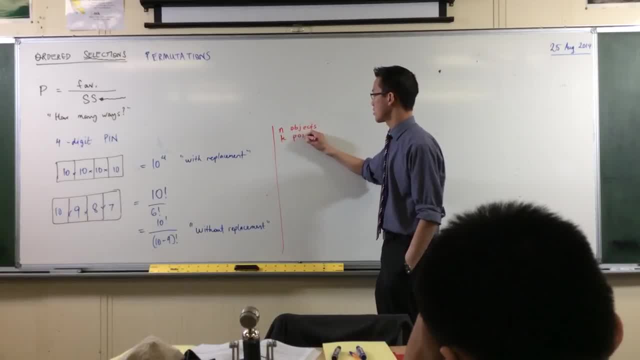 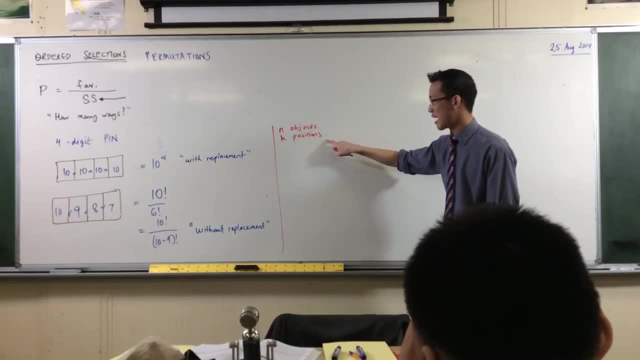 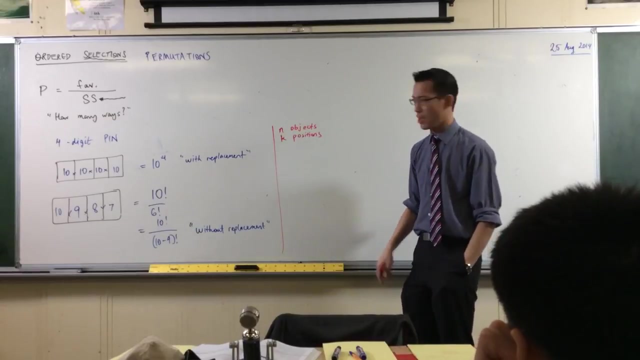 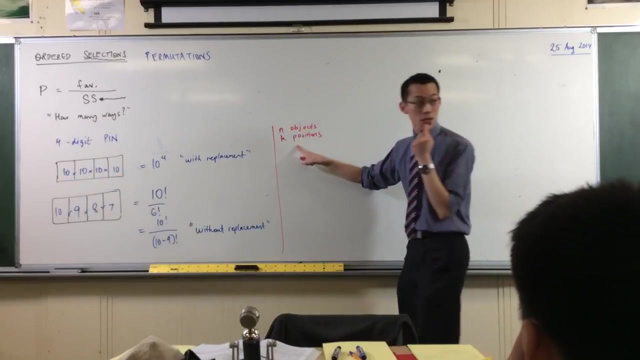 Okay, And I have k positions to put them into. Okay. If I have n objects and I want to put them into k positions, Okay. Then in this case, how many permutations are there? Well, it'll be n times n times, n times n, however many times you have positions. 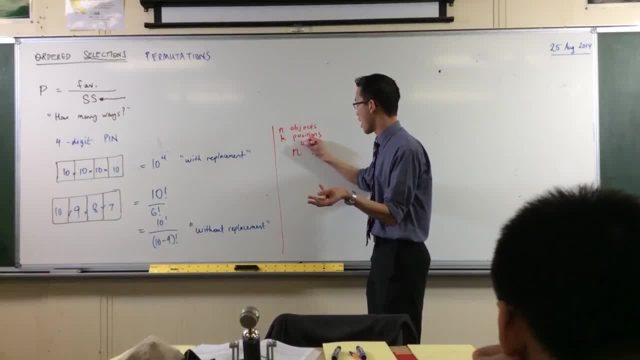 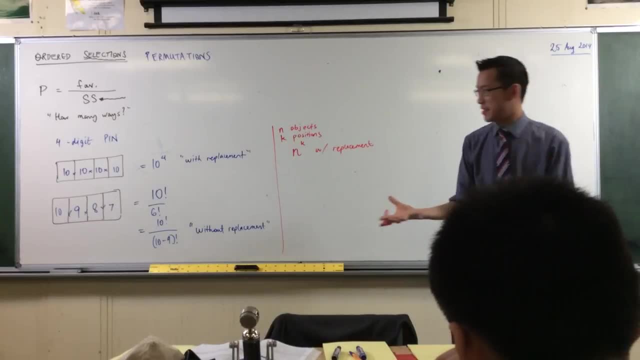 Right K times. So that would be n to the power of k with replacement. Okay, Obviously you could expand this out to say: you know what if it wasn't numbers? What if we allowed letters in there as well? 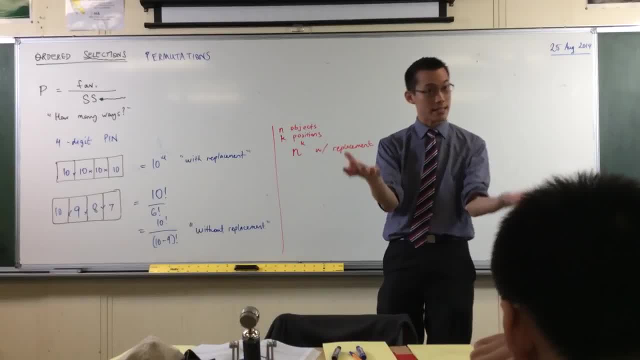 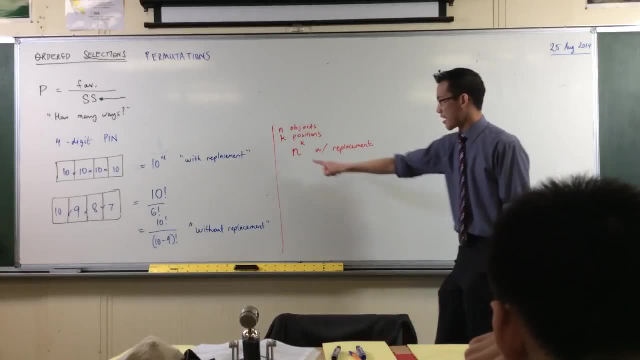 And then I guess you would have your ten digits and your twenty-six letters And you would say: well, it would be thirty-six to the power of four Obviously minimal options, Right, Okay. Now, when you come down to here, it's a little more complicated, but it's still the same. 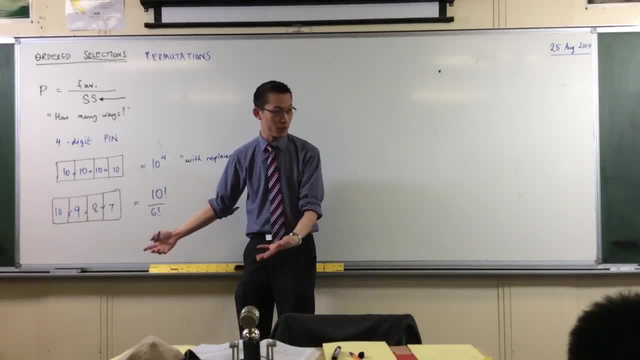 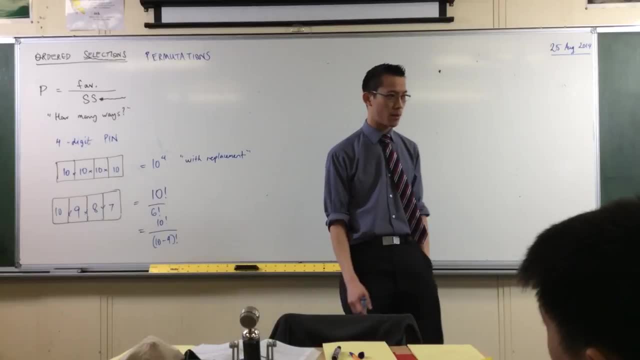 So that's why there are six factorial left over here that I haven't included, right? So it's ten factorial on ten minus four factorial. That's really where the numbers come from And you can see it's built of the same numbers as this, right. 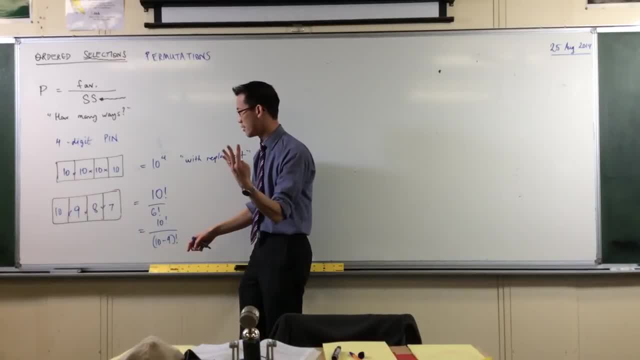 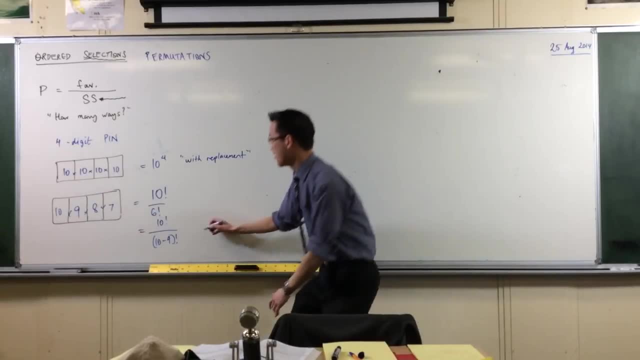 The ten, as in how many digits there were. and the four- sorry, Ten, how many different numbers you could choose from. And four, how many digits there were. That's how we built this number of permutations. okay, So this is without replacements. 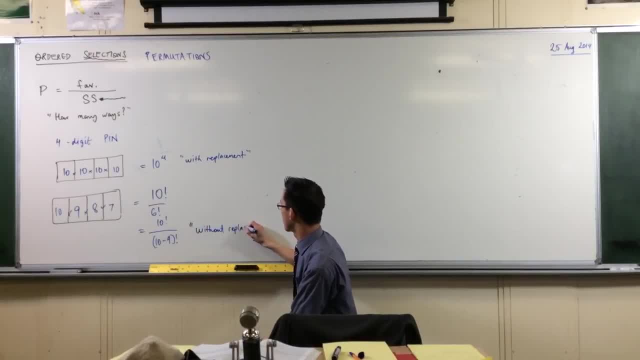 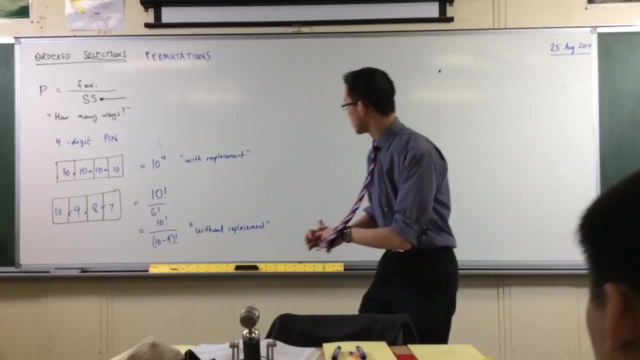 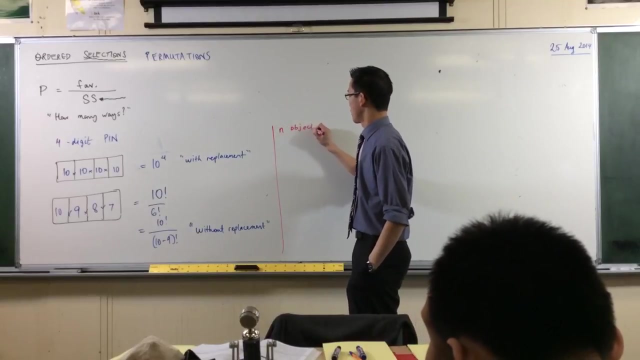 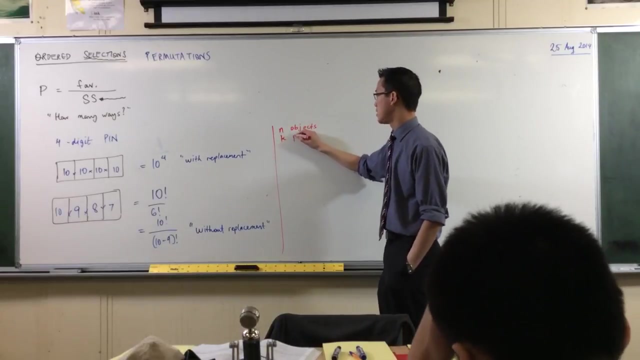 Okay. so let's generalize a little bit. If I have- let's put it over here- okay, if I have n objects, n objects, for instance, if I have ten numbers: 0,, 1,, 2,, 3,, 4,, 5,, 6,, 7,, 8,, 9,, okay, and I have k positions to put. 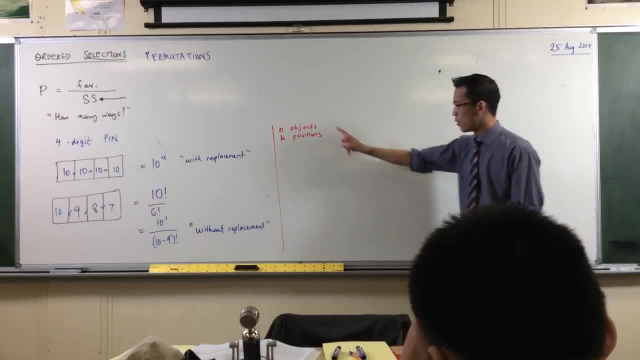 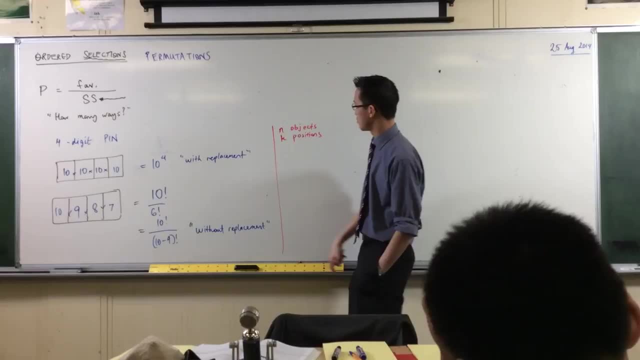 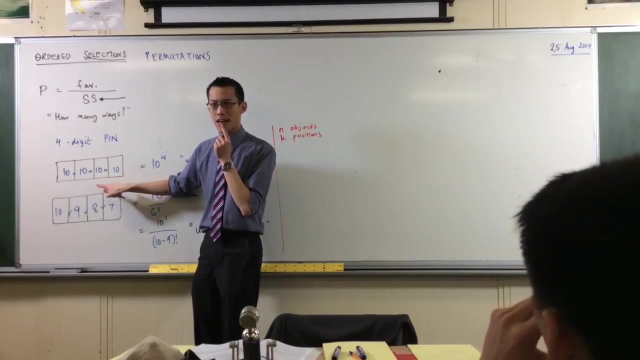 them into, okay, If I have n objects and I want to put them into, okay, Okay. Okay, Then, in this case, how many permutations are there? Well, it'll be n times n, times n, times n, however many times you have positions right. 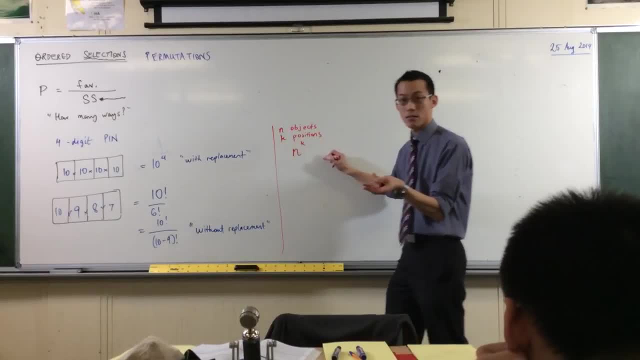 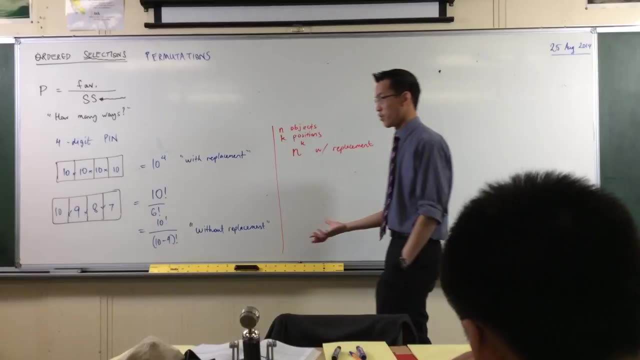 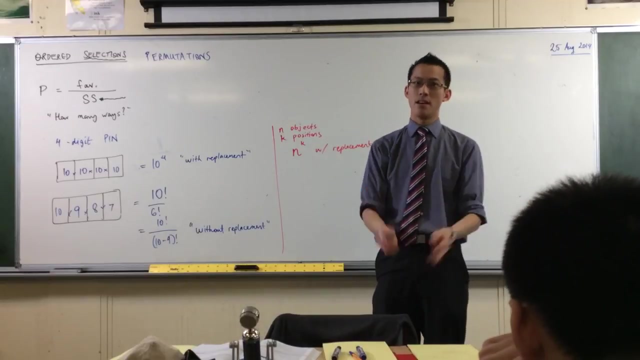 K times. So that would be n to the power of k with replacement. Okay, obviously you could expand this out to say: you know what if it wasn't numbers? What if we allowed letters in there as well? And then I guess you would have your ten digits and your twenty-six letters and you would 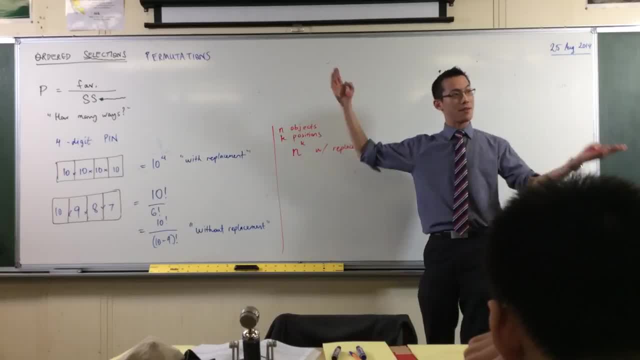 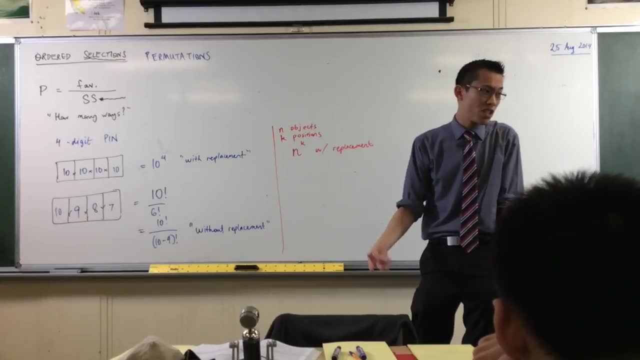 say: well, it would be thirty-six to the power of four- Obviously minimal options, right, Okay, now, when you come down to here, it's a little more complicated, but it's still the same numbers. It's still the same numbers. 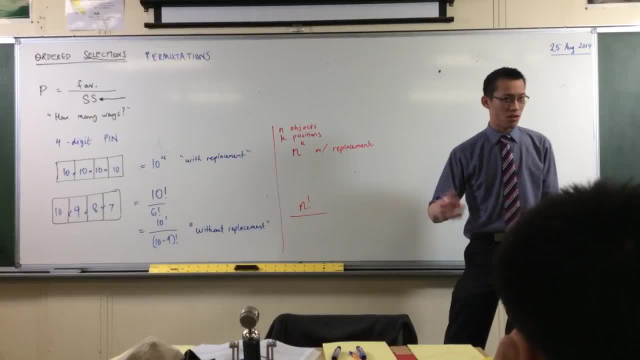 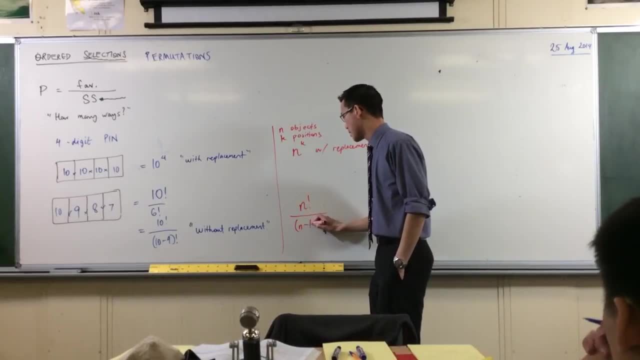 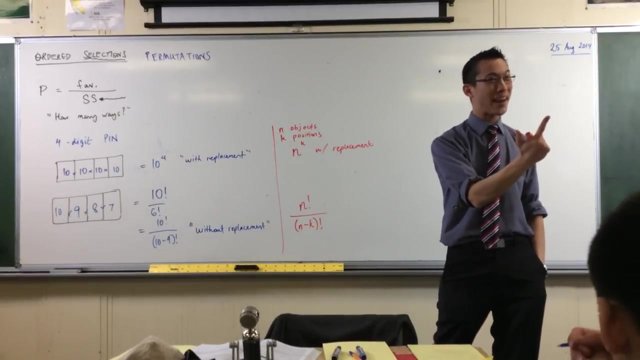 You're still going to have n factorial to start with, but you're not going to have n factorial by the end, unless you're picking that many positions right. I've got k positions, So this would be n minus k. Now this comes up so much and it's so awkward to put into your calculator repeatedly that 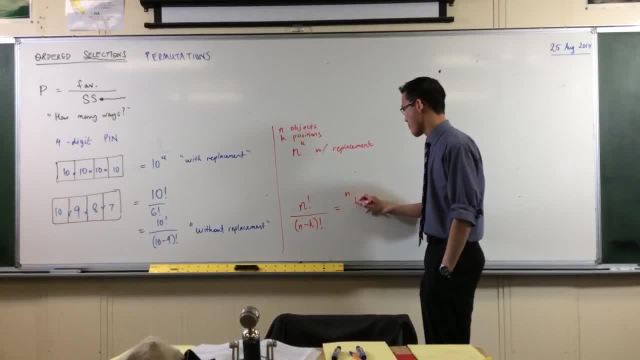 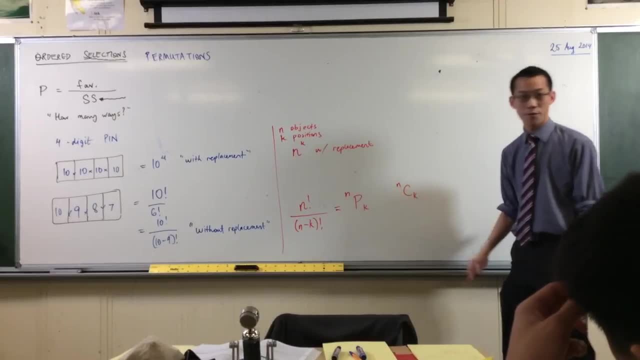 your calculator has a special button for this. We say it's n p k And it's right next to its important cousin, which you're familiar with. you're more familiar with n c k. We'll come back to this guy in future times because I know you're familiar with him. but 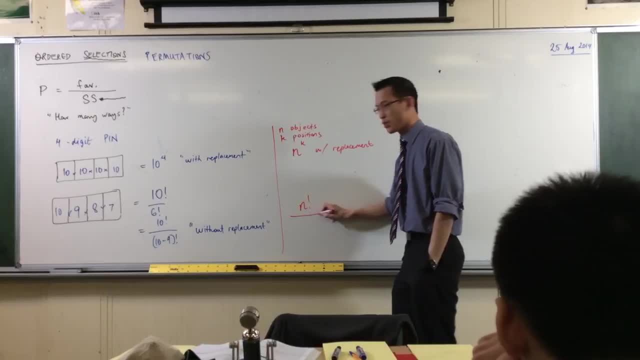 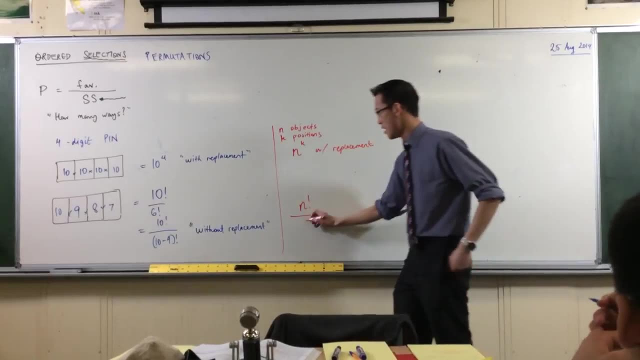 numbers. It's still the same numbers. You're still going to have n factorial to start with, but you're not going to have n factorial by the end, unless you're picking that many positions Right. I've got k positions. This would be n minus k factorial. 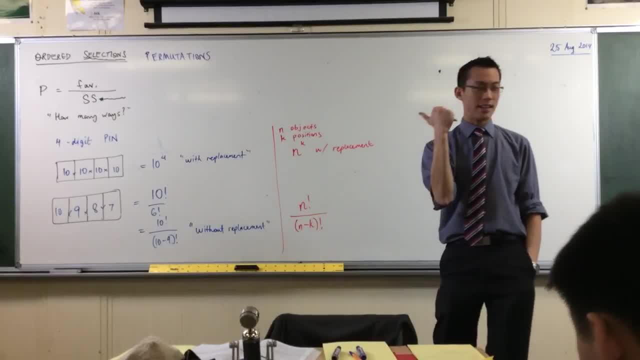 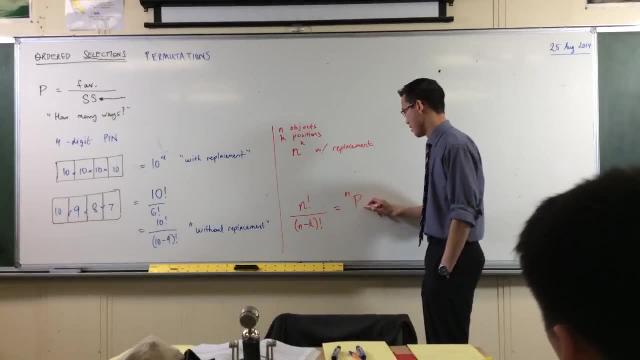 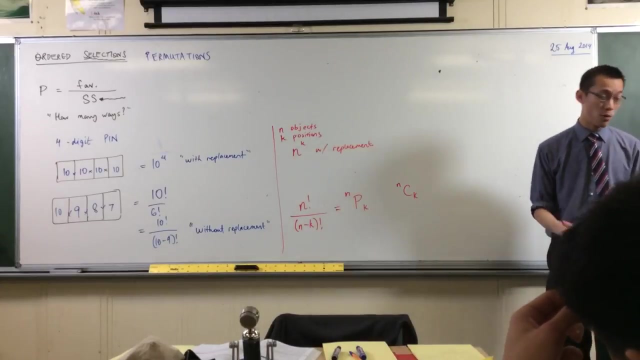 Right Now this comes up so much and it's so awkward to put into your calculator repeatedly, that your calculator has a special button for this. We say it's npk And it's right next to its important cousin which you're familiar with. you're more familiar. 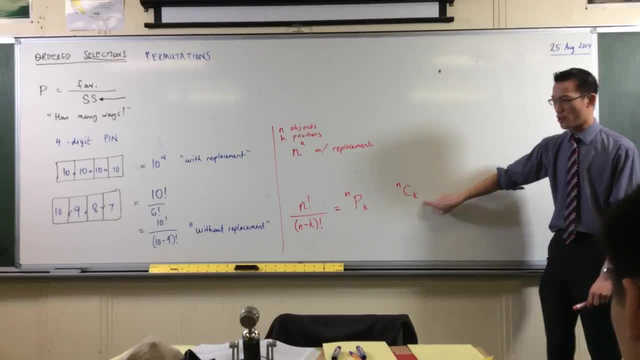 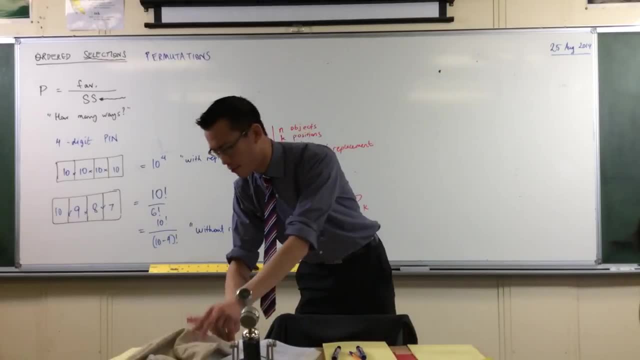 with nck. We'll come back to this guy in future times because I know you're familiar with him, but he comes up in this context a little differently. Okay, So I think it's shift. what is it above? Is it above like plus or minus or something? 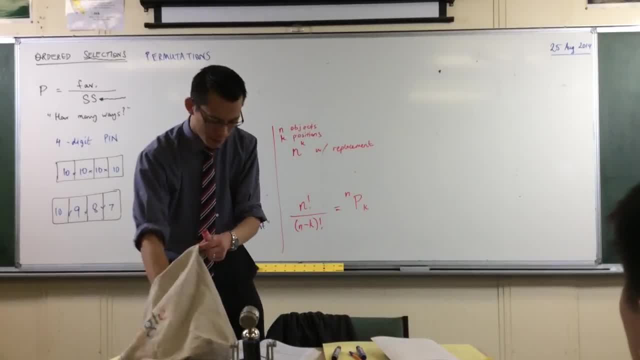 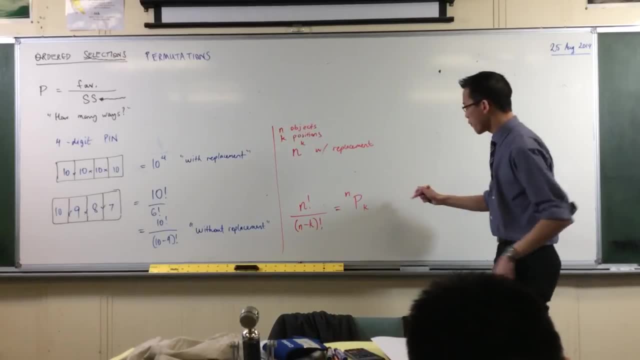 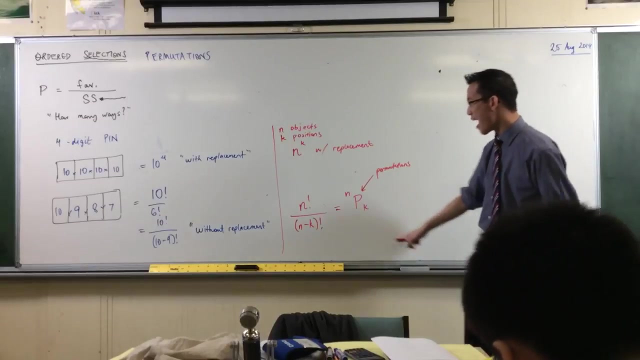 Times Plus Times. So you've got p for- yeah, it's above times, It's p for permutations, really. But just in normal language You either say npk or you say npk, K, Okay, K. 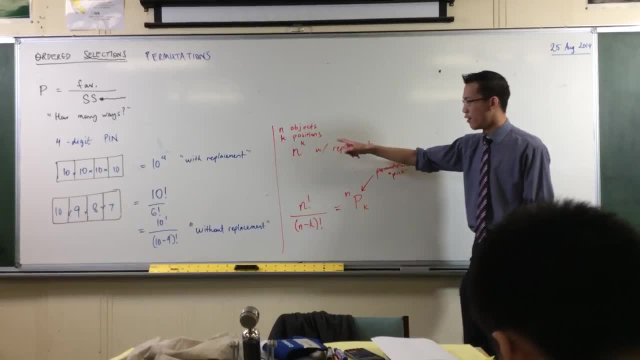 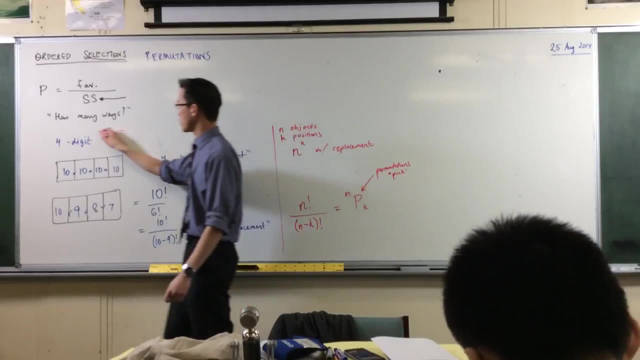 Right, Because I want to pick out k of them. I want to pick out four of them, Right, And I've got n to choose from. Does that kind of make sense? And this scenario, like the four digit pin, it comes up again and again, and again. 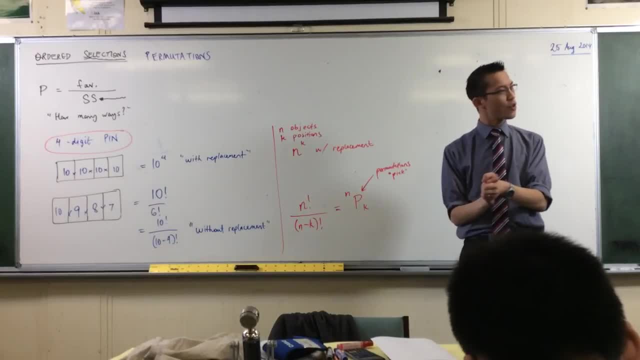 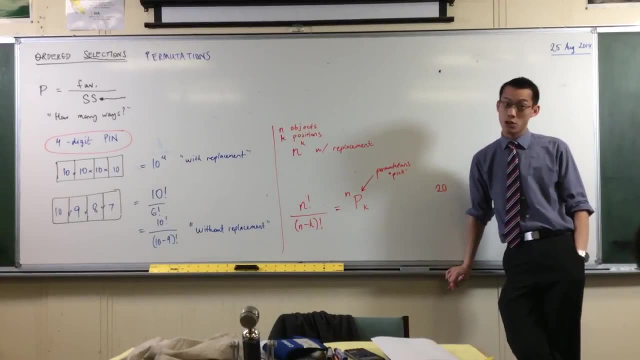 You've got 20 horses in a race. How many different trifectas are there? 20 horses in a race, 20 horses Right? Is this with or without replacement? It's a trifecta. A trifecta is first, second and third place. 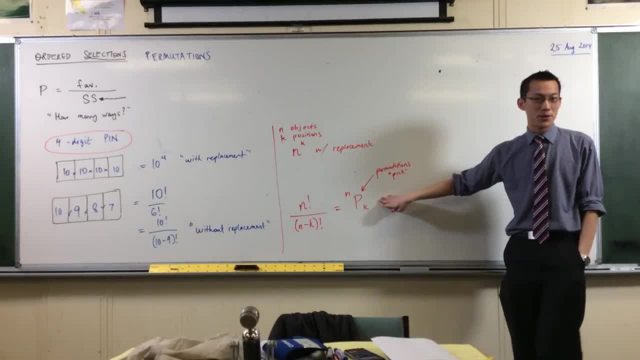 Right. Clearly that's without replacement, because you can't get the same horse coming first and second and third, unless it's some kind of weird quantum Schrodinger's horse or something I don't know Anyway. So you've got 20 to choose from. 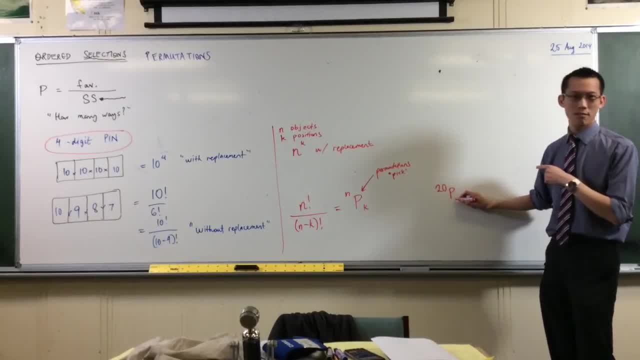 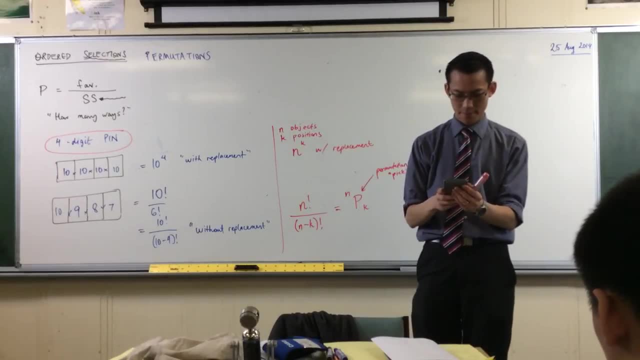 It's without replacement. It's this scenario, Right, So you're going to pick three: 20, pick three. By the way, what is 20, pick three? I assume it's a very large number, 6. 6.. 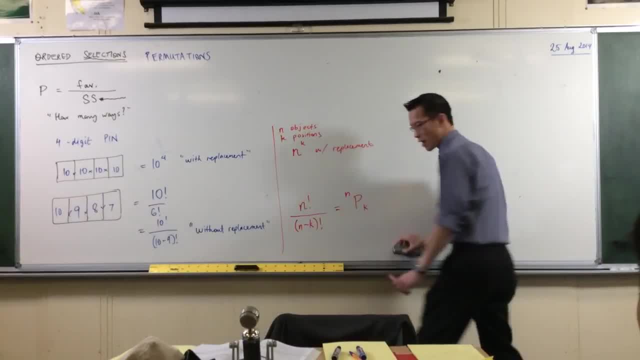 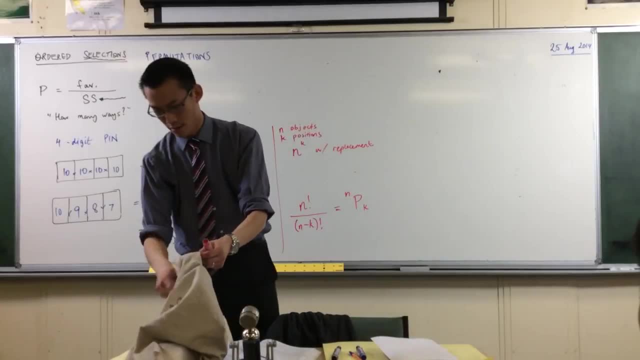 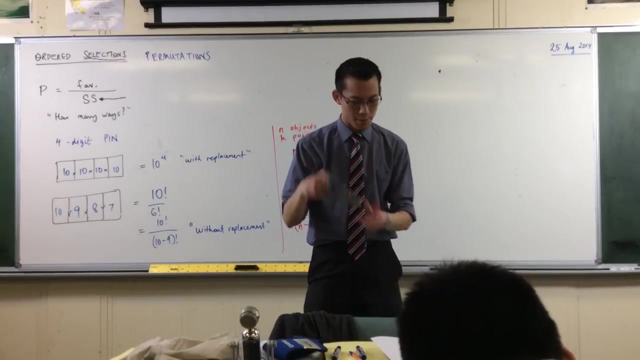 he comes up in this context a little differently. So I think it's shift. what is it above? Is it above like plus or minus or something? Times Plus Times. So you've got p for yeah, it's above times. 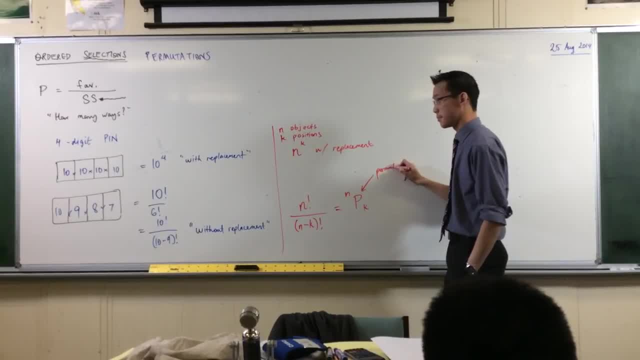 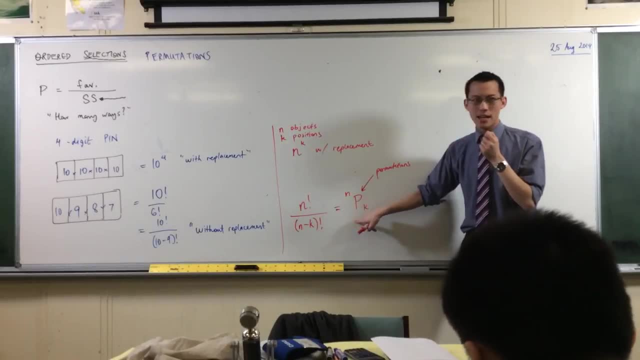 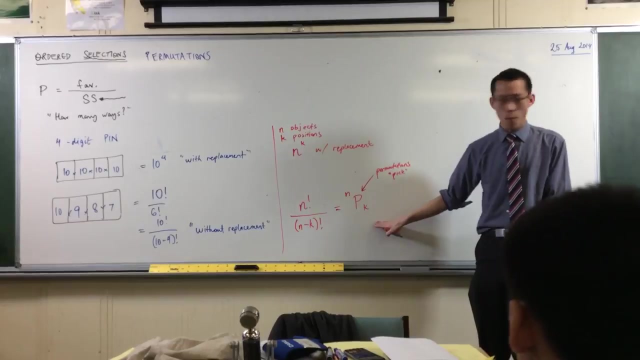 It's p for permutations really, But just in normal language you either say n p k or you say n pic pic k, right, Because I want to pick out k of them. I want to pick out four of them, right. 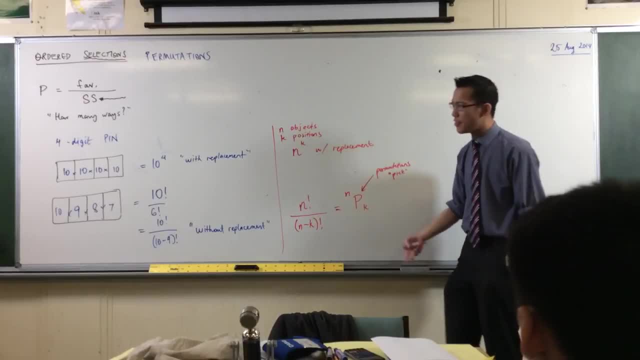 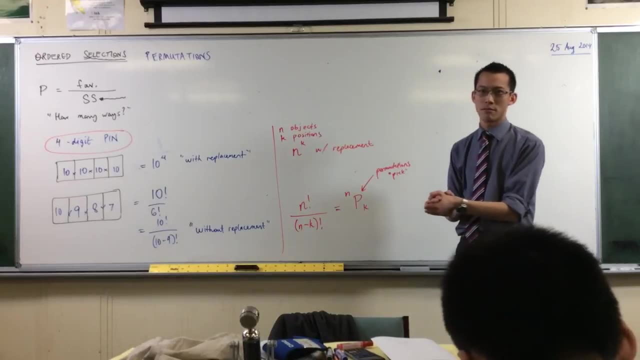 And I've got n to choose from. Does that kind of make sense? And this scenario, like the four digit pin, it comes up again and again and again. You've got 20 horses in a race. How many different trifectas are there? 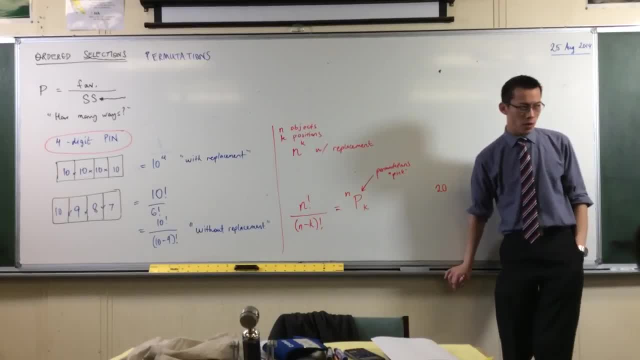 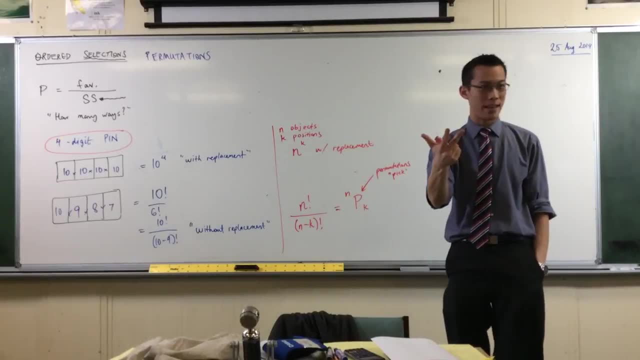 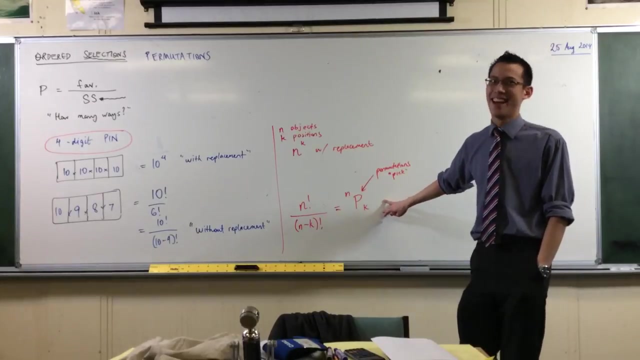 Twenty horses in a race, twenty horses right? Is this with or without replacement? It's a trifecta. It's trifecta is first, second and third place right. Clearly That's without replacement, because you can't get the same horse coming first and second. 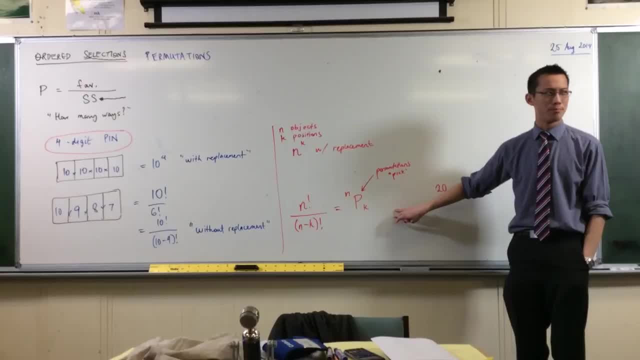 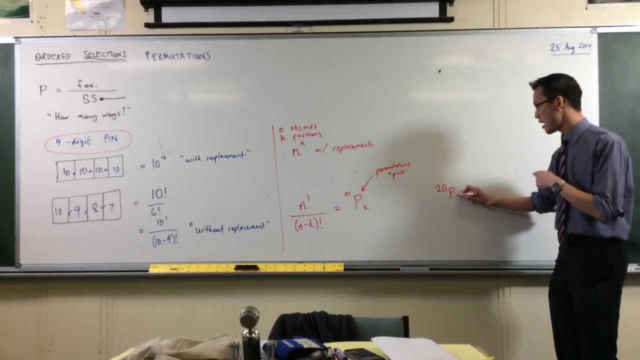 and third, unless it's some kind of weird, weird quantum Schrodinger's horse or something, I don't know Anyway, So you've got twenty to choose from. It's without replacement. It's this scenario, right? So you're going to pick three. 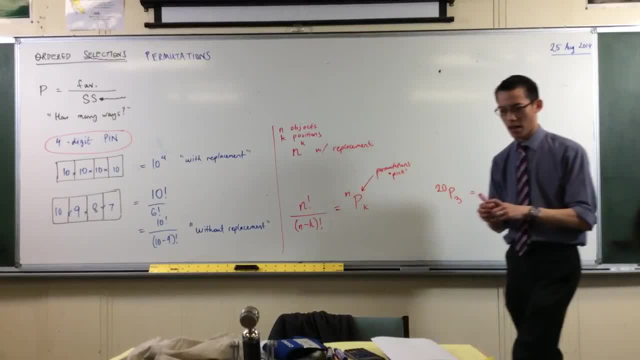 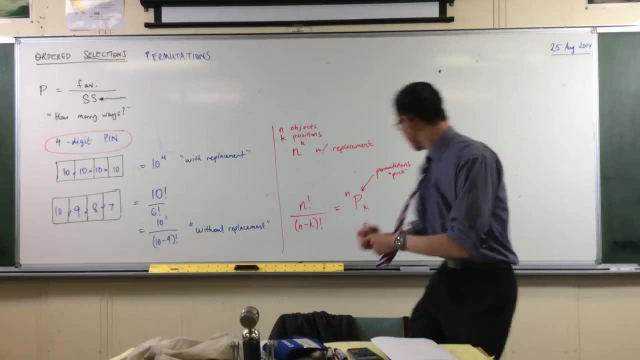 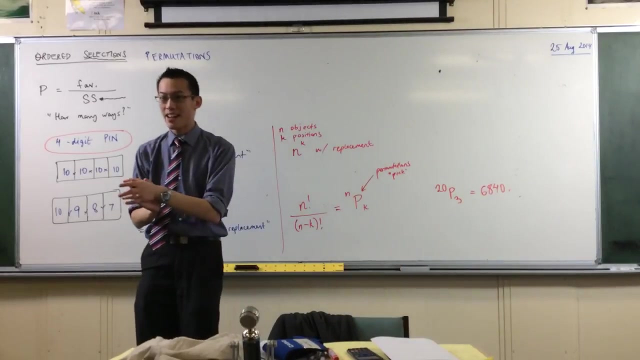 Twenty pick three. By the way, what is twenty pick three? I assume it's a very large number: Six thousand eight hundred and forty Right Right. So if there's a twenty horse race and you're betting right and a trifecta is a thing that, 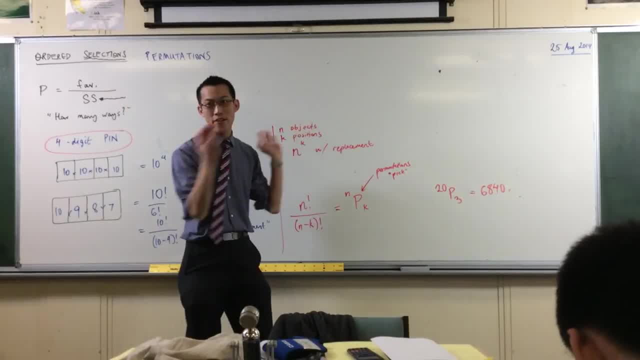 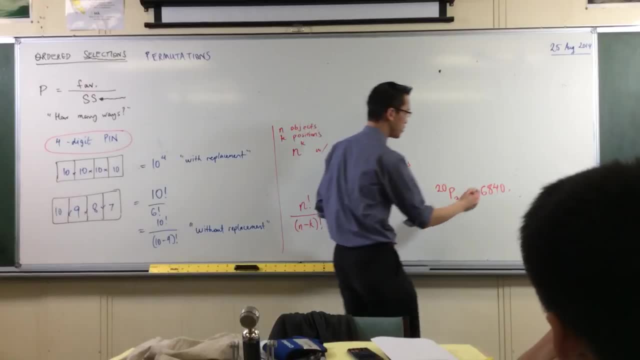 you bet on right if you don't know anything, and you pick out a trifecta at random right which, by the way, if you go, if people go to the TAB and they'll just press like a random generator because like, oh, who knows right, well, that means you've got a one in. 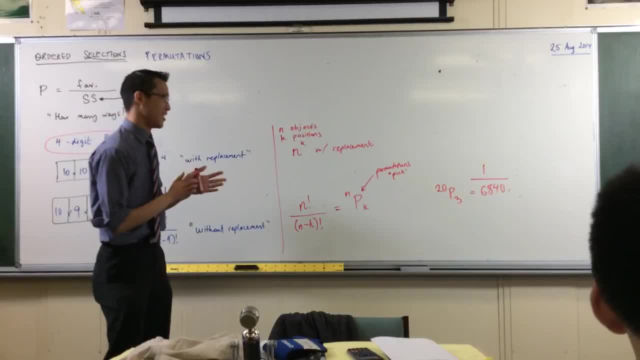 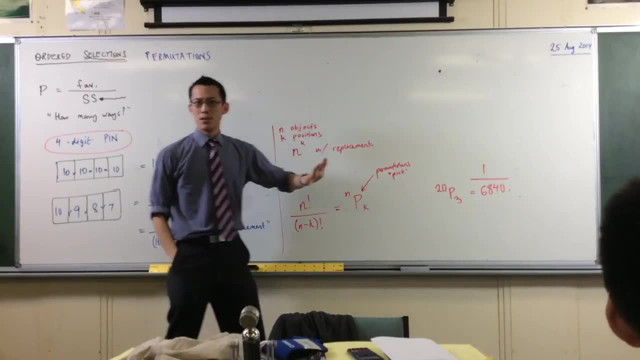 Six thousand eight hundred and forty chance of getting the trifecta. I think I'd rather go wash a car and ask for ten dollars if I want to earn money. but anyhow, each to his own. So does that make sense? Yeah? 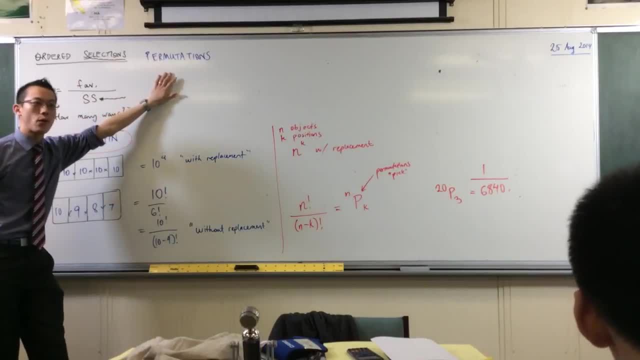 So there are two ways of approaching permutations, based on whether you're replacing or not. Most liquids, when cooled, will simply shrink. Water, on the other hand, actually expands. when it is frozen, Its volume will increase by about 9%. Suppose you have 1 third of a gallon of water that gets frozen. What is the volume of the ice that you now have? 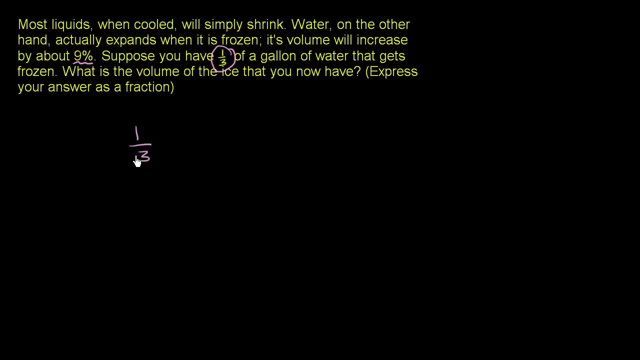 So you're starting with 1 third of a gallon of water And they tell us that when it gets frozen, when it turns into ice, its volume is going to expand by 9%. So the new volume is going to be your existing volume. 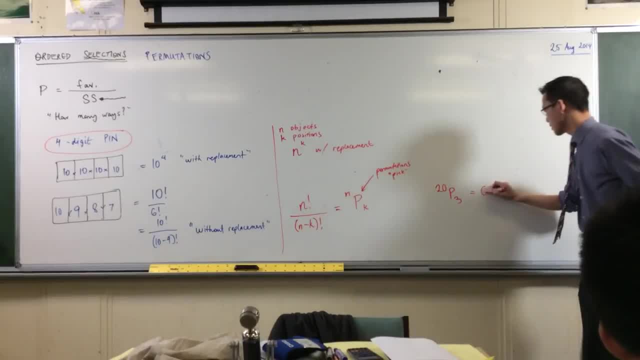 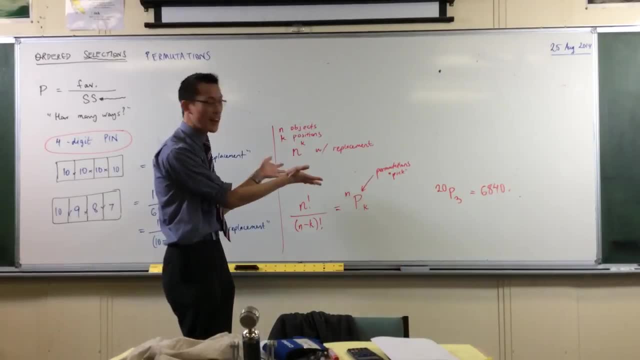 6,840.. 6,840. Right. So if there's a 20 horse race and you're betting, right and a trifecta is a thing that you bet on, right. if you don't know anything and you pick out a trifecta at random. 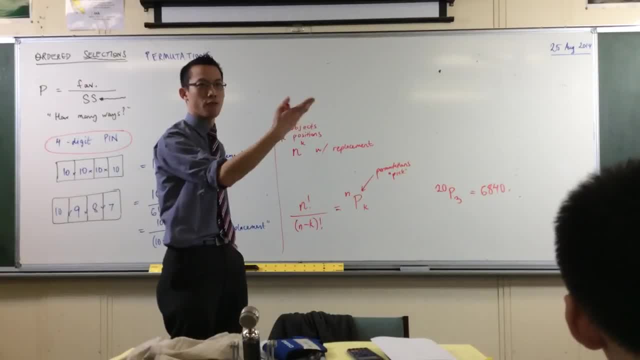 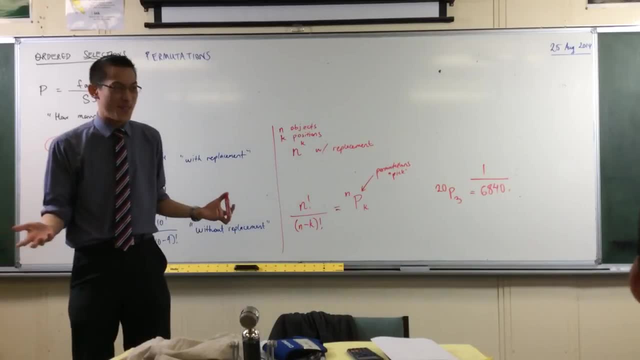 right, which, by the way, if people go to the TAB and they'll just press like a random generator, because like oh, who knows right, well, that means you've got a one in 6,840 chance of getting the trifecta. 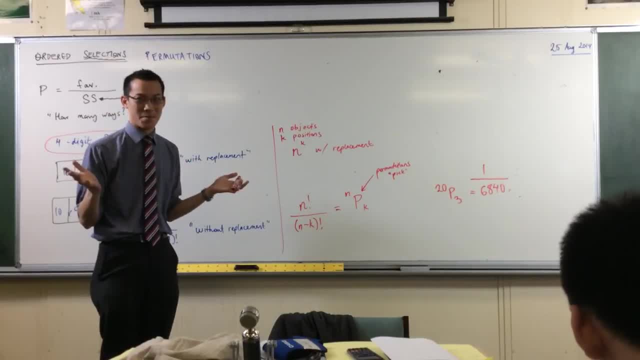 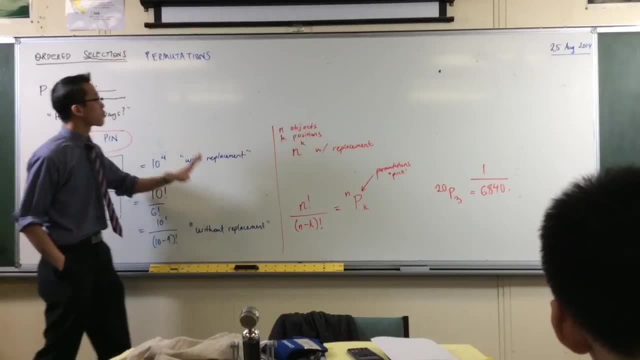 I think I'd rather go wash a car and ask for $10. If I want to earn money, But anyhow, each to his own. So does that make sense? Yeah, You've got these two ways of approaching permutations, based on whether you're replacing. or not. 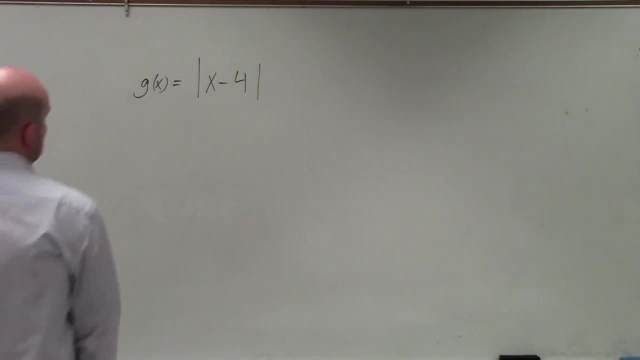 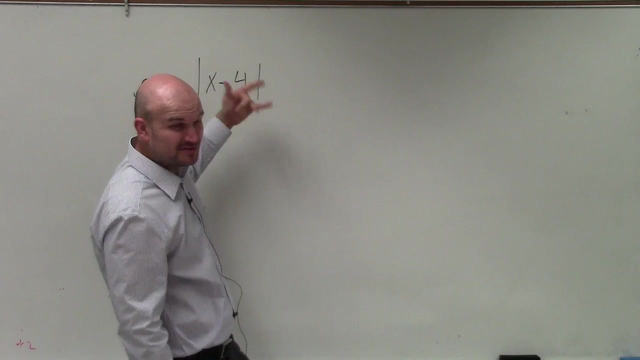 So once you guys go ahead and graph this, hopefully you guys have understand- if you guys remember from your notes last class period- when you are subtracting a number inside of the function, it's inside the bracket, so it's inside the function that's shifting the graph four units to the right. So 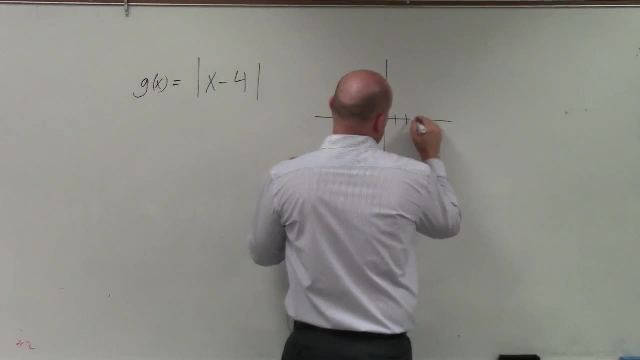 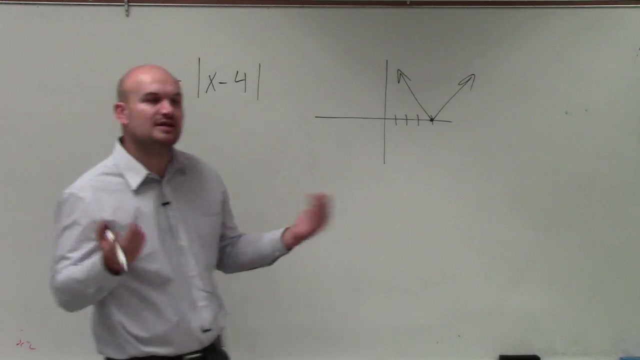 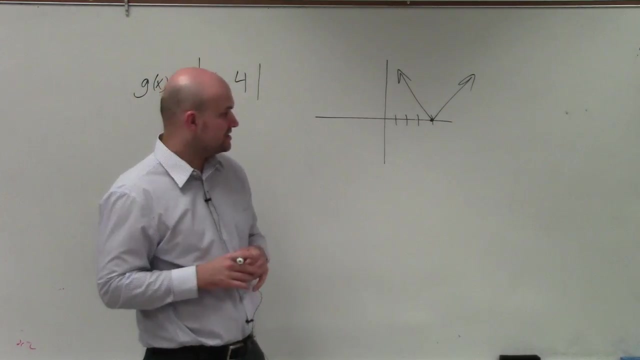 typically, you have your absolute value function, which is now just being shifted four units to the right, So your graph should look something like that, right? If not, make sure you guys go to zoom standard and hit zoom and then go to option 6, which is zoom standard, and you should see something just like that Now. 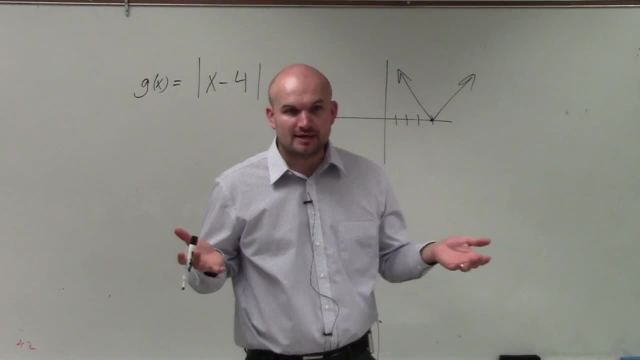 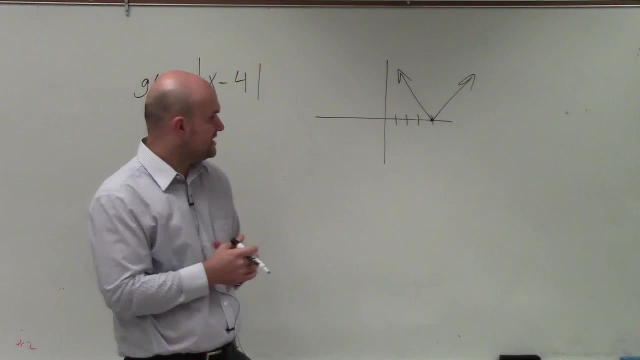 I want to talk about the domain, because we've talked about the domain algebraically right Finding and basically finding the domain algebraically. we just look for when was the function not in the domain and we wrote that in interval notation. Well, when we're looking at the graph, 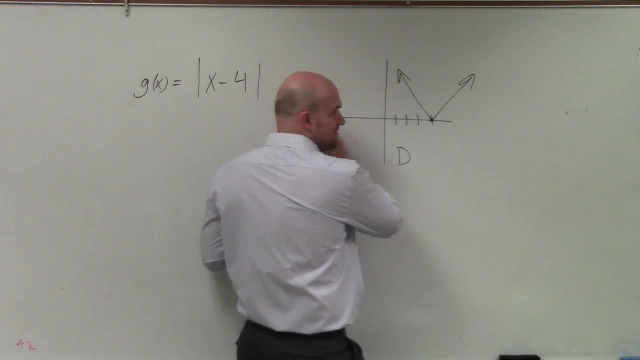 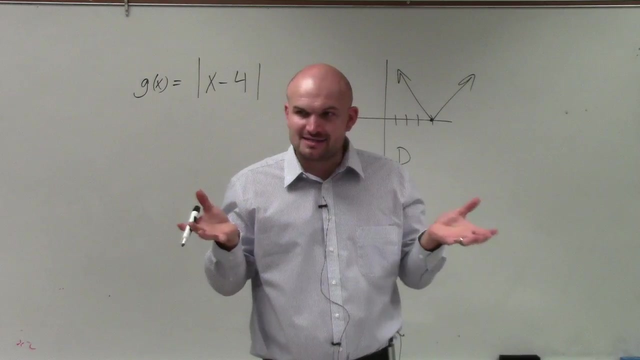 basically finding the domain is: how far does graph go to the left, how far does graph go to the right? So even if you are on a test, you could always graph a function and visually look at it to kind of verify. make sure you algebraically,